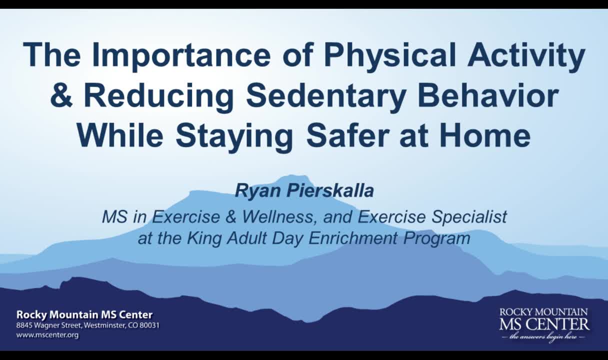 to Ryan. Thanks, Kelsey. Hey there everyone. I'm Ryan And, as Kelsey mentioned, I'm over at KDEP. I've been there about two years now And, yeah, during normal times I lead exercise groups. 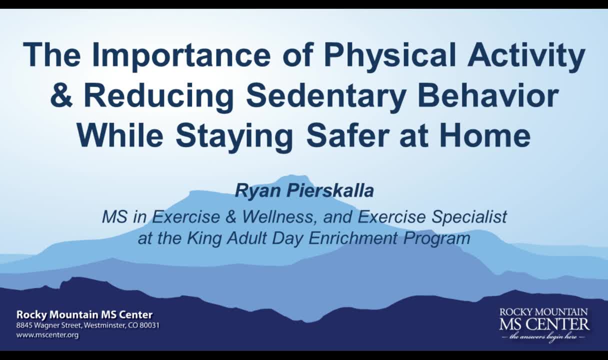 out of our fitness center And I'm also a member of the KDEF. So I'm a member of the KDEF. I also do weekly hydrotherapy with a group of clients where we go throughout our surrounding community rec schools. That's during normal times. We're limited at the moment But in 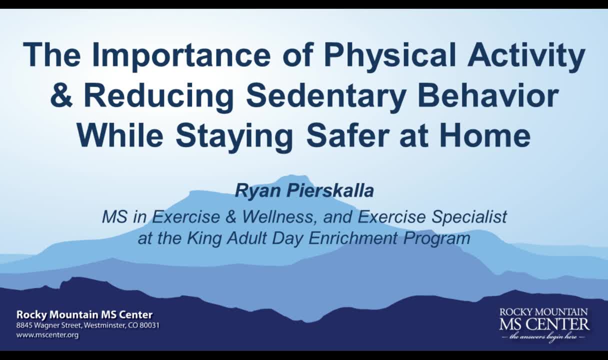 both arenas. my goal is to deliver physical maintenance and improvement. I'm a Colorado native. I got my degree, as Kelsey said, from Colorado State, with Arizona State for the Masters And then came back here to Colorado, where I belong. So with that in mind, we'll 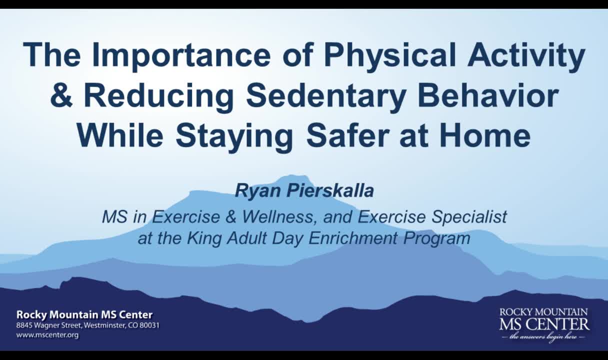 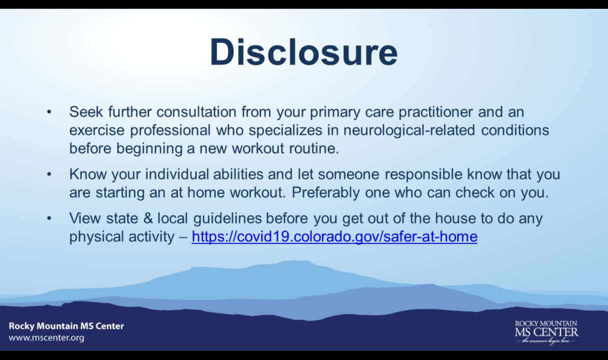 take a break, And today I'd like to talk about the importance of physical activity and reducing sedentary behavior while staying safer at home. So just a quick little disclosure here. Be sure if you start any new regimens of physical activity, if you're really just jumping in. 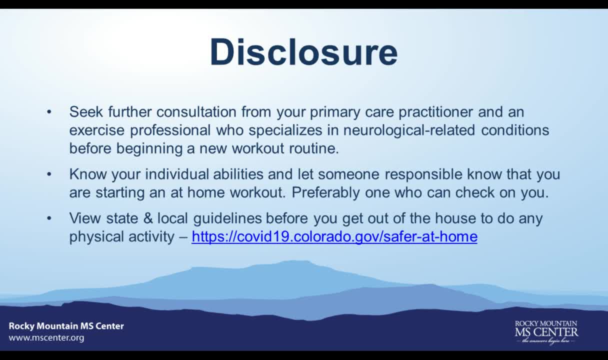 for the first time, especially seek further consultation from your PCP and an exercise professional who specializes in neurological-related conditions before beginning that routine. Know your individual abilities and let someone responsible know that you are starting an at-home workout, preferably someone who can check in on you as in a family member. that 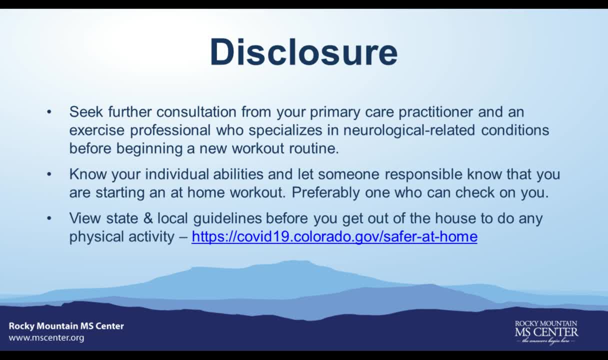 lives with you or whoever is there at the home you know is responsible. View state and local guidelines before you get out of the house to do any physical activity. Great source that we found is through coloradogov, listed there: covid19.coloradogov backslash. 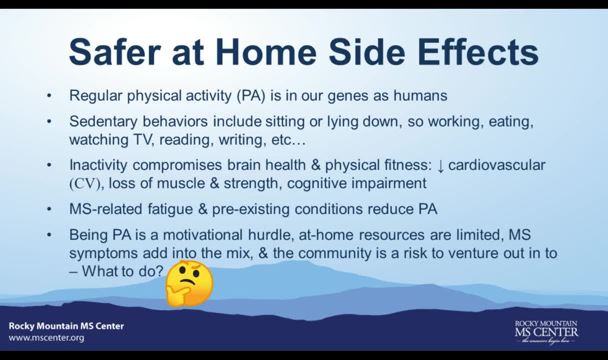 safer at home. So the issue at hand that we face right now- safer at home orders- and we have we're facing safer at home orders and restricted access to gyms, schools and fitness centers. It's all been very limiting and has drastically affected physical activity and exercise. 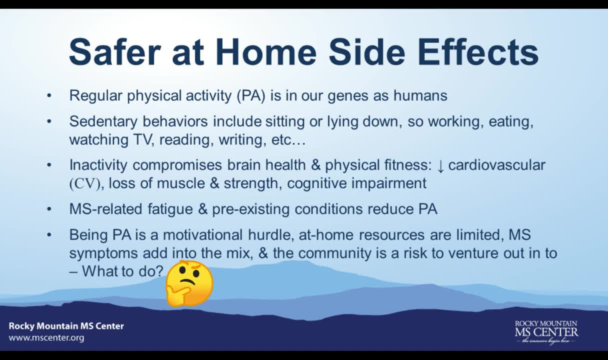 Also, social distancing and hygiene are currently the best and only methods to limit the spread of the virus. As everyone has found out over the past few months, this is incredibly limiting in several ways, especially with our physical health. Everyone is having to steer clear of contracting virus by staying safe at home and physical 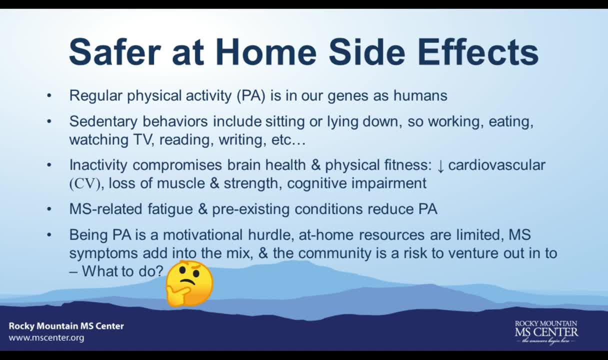 activity and mental health. Medical health is suffering in this process, Same as animals. however, humans need physical activity. it's in our genes. Just think about how much running around your dog does compared to you. That analogy should give you some perspective, unless you have a lazy blue heeler mix who. 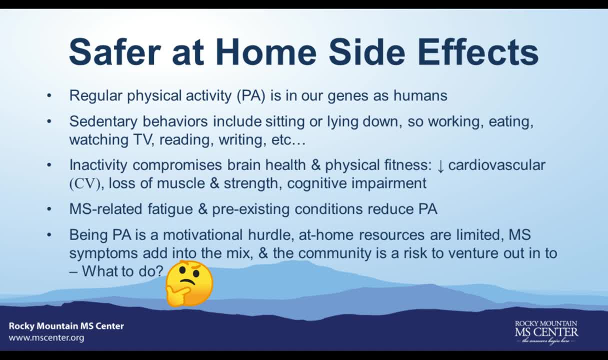 thinks she's a human, like my family's dog, Piper. However, she is living Piper's living her best life as my parents, as they work from home and Set and trade. behavior is very important. Behavior is classified as sitting or lying down, so all of the above that we can think. 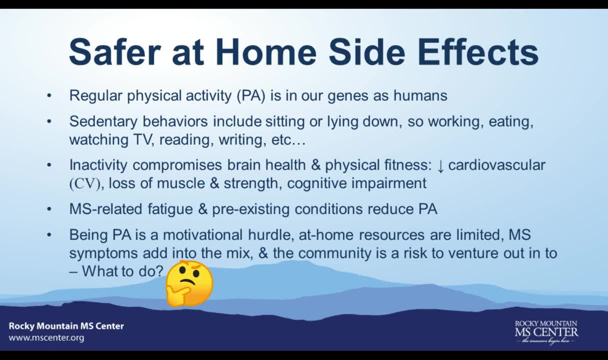 of, as in working at a seated desk, eating, watching TV, et cetera. this affects physical fitness and forms of cardiovascular or heart health, as well as strength and muscle loss. I'll break these down a bit more in some later slides. 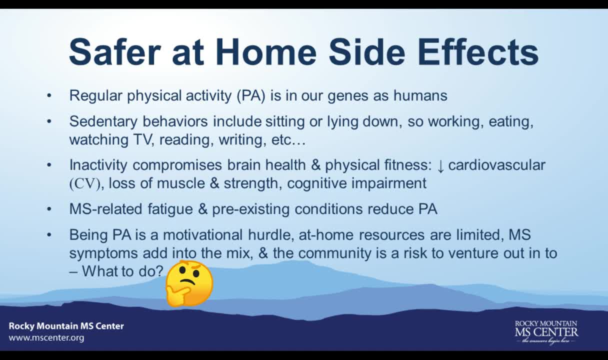 Plus, inactivity and isolation compromises brain health, as in impaired cognition and thinking skills. With our Rocky Mountain MS Center population, they are having to deal not just with fatigue from increased bouts of inactivity but from pre-existing local sclerosis or other neuro-related 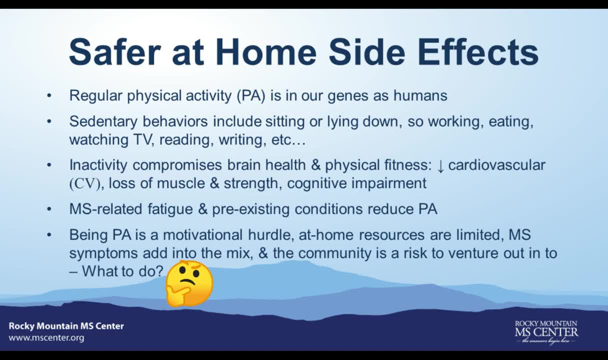 conditions or disorders. Physical activity, likely, was already a challenge for this population, with their varied symptoms and severity of multiple sclerosis, Now even more confined in a new lifestyle, In this new lifestyle that we face, where we're constantly at home, symptoms of inactivity. 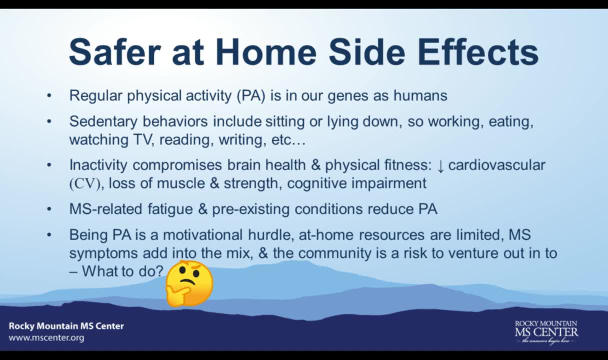 and MS, along with decreased motivation, can all become even more exaggerated. With all these hurdles, what do you do? I'll try to break a few of them down and give some meaning to a few of these, so you can hopefully get some insight and a different perspective. 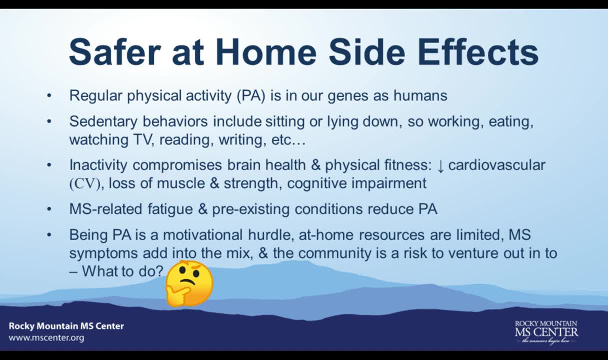 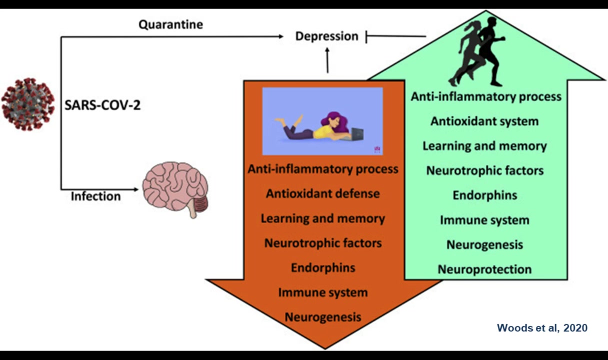 Thank you. Thank you, Let's see. Okay, So this figure from a recent study done by Dr Jeffrey Wood and his colleagues at the University of Illinois related to the pandemic and physical activity, that's what the figure is here. COVID-19 is the effect caused by the severe acute respiratory syndrome, coronavirus 2 or 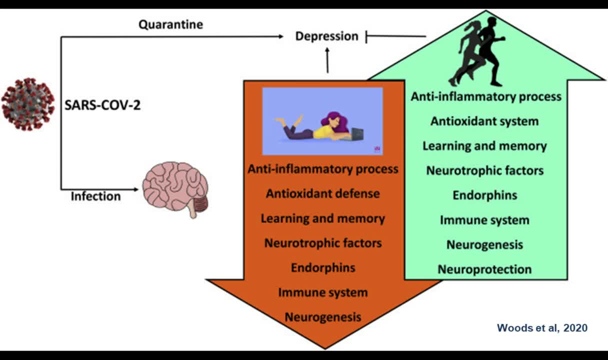 SARS-CoV-2.. The rules are out of the tongue. This can directly attack the central nervous system. quarantine to prevent the spread of SARS-CoV-2 can lead to depression, while being cut off from other people and from a substantially. 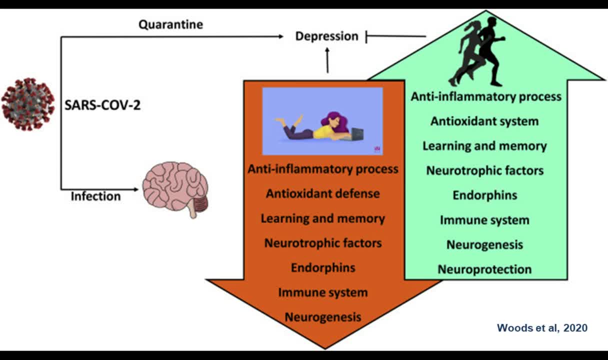 healthier or unhealthy routine. This further infects the central nervous system and the immune system. Other factors leading to depression are listed there in the negative orange arrow, and they are also responsible for signs of depression seen during quarantine. However, regular physical activity performed at a moderate intensity while quarantined- 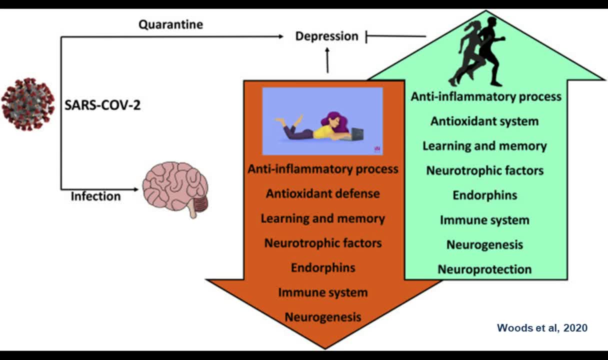 can curb or alleviate these symptoms shown by the positive happy green arrow. Also, it helps to block off any state of depression. essentially, One more little figure from that study on COVID-19.. This figure relates to older adults who had been exposed to COVID-19, and they're at a 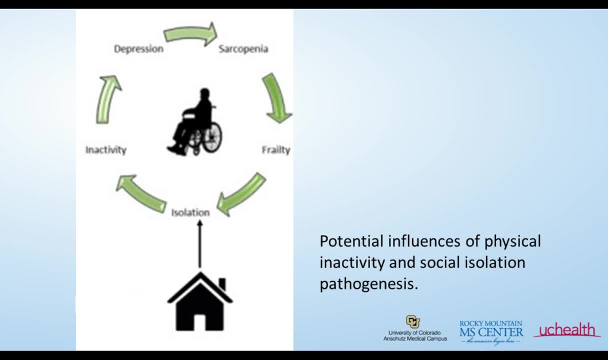 different level of risk than younger individuals, or maybe people just with MS, but still worth noting the cycle from isolating for such long periods of time. The figure also adds an important term to keep in mind here for my presentation is sarcopenia. 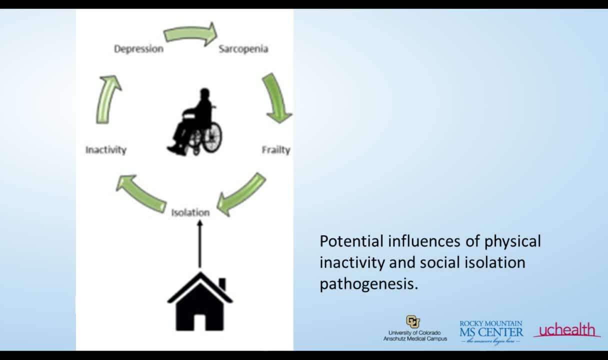 which means that a person who has been exposed to COVID-19 for a long period of time is at risk of getting COVID-19.. This figure also adds to the decline in muscle with regards to mass and quality, and that leads to strength loss, lecture balance and a bunch of other things. 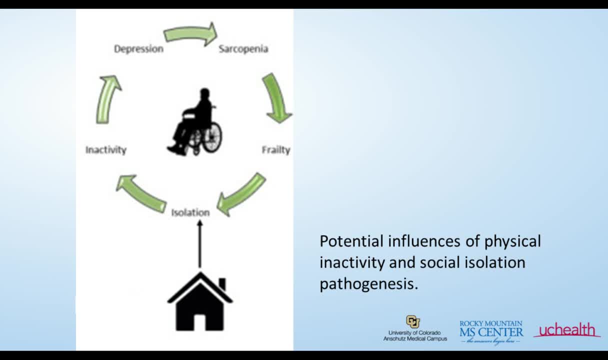 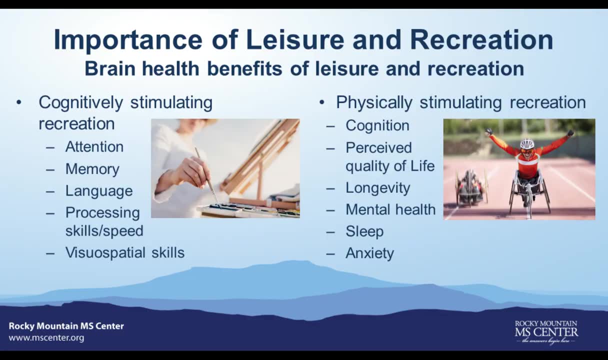 So earlier in April, my programming director, Emily Nelson, talked about the benefits of recreation and leisure activity As it pertains to now safer at home orders And to this series of brain health webinars. Emily talked a bit on brain health benefits. 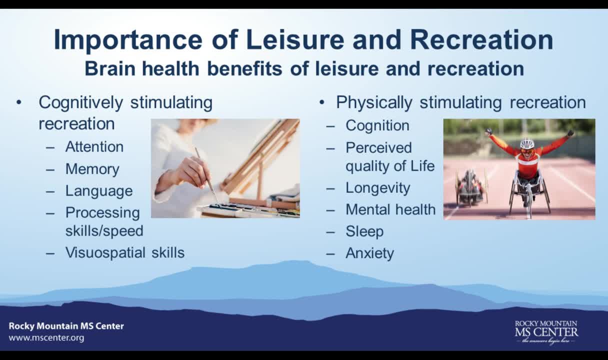 as we hear from cognitively stimulating and physically stimulating recreation therapy. The importance of this, as it relates to the webinar, is cognitive function is inversely related to physical activity. They share a connection for the release of endorphins, dopamine, serotonin and norepinephrine. 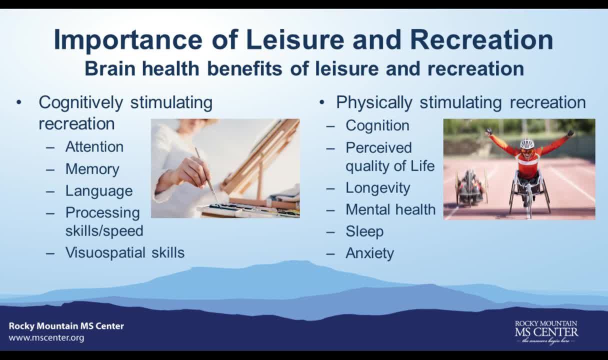 released from the brain. They also help to improve mood and mood control during recreational activities and boost mood and mental health. Then the stimulating- excuse me, then the stimulated- cognitive pathways can return the favor to promote more physical activity. It's like a John Krasinski-esque circle of some good news and positive reinforcement. 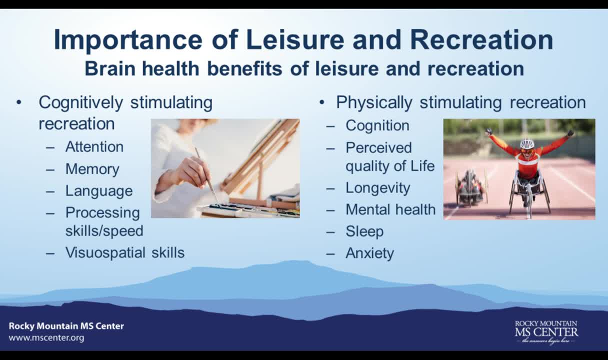 between physical health and mental health where they can feed off of one another. Keeping on with the importance of physical activity, I will quickly mention that I am lumping in leisure activity, recreation exercise, working out anything low or moderately intense that requires some energy expenditure or mental 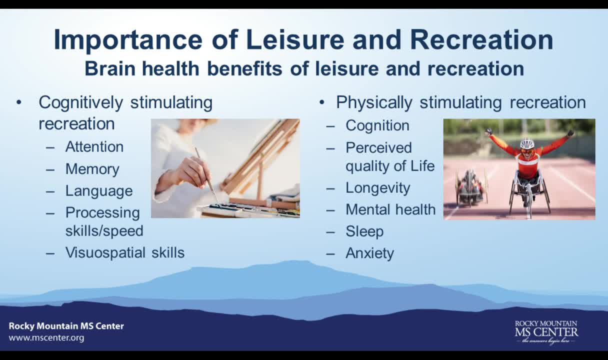 power, as physical activity accounts towards your physical health in kind. The reason physical activity is important to the clients and patients who are part of the REC 9-MF center are the ones listed here: The heart health we've mentioned And weight management, where you can potentially hold at a number but not significantly lose. 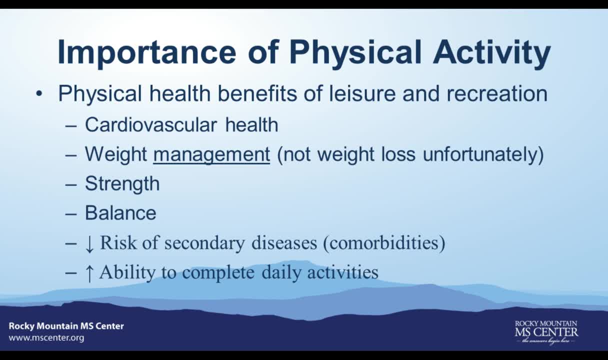 weight. unfortunately, Losing weight, that depends on calorie intake, metabolism, genetics and a bunch of other factors I won't get into here. But physical activity will still help you at least to maintain your weight. Other benefits, you see there are improved strength and balance, along with decreased 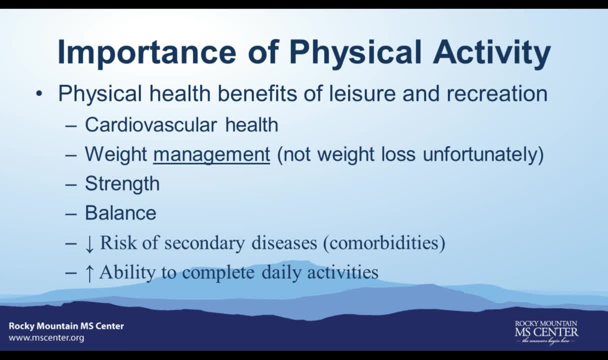 risk of secondary diseases, also known as comorbidities, and a great functional ability to complete your everyday tasks. And let me make it clear and not pull a disinfectant vaccine type of gap: I mentioned right now that physical activity won't prevent the disease for you from contracting. 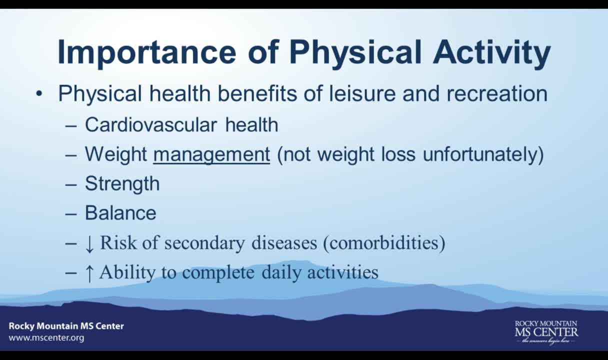 the virus. It's certainly not a vaccine, but it can potentially help boost your immune system to protect against and lessen the impact of the symptoms if you do contract it. And, yes, physical activity has shown to help. I'm sorry. I'm sorry. 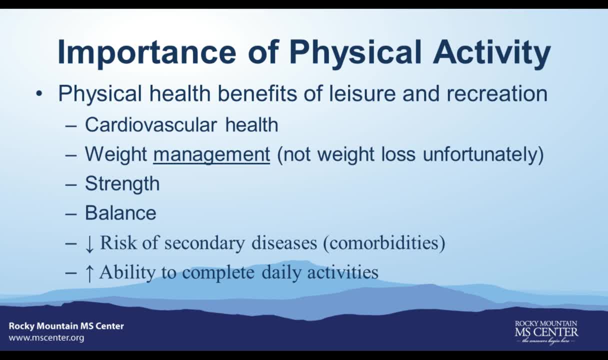 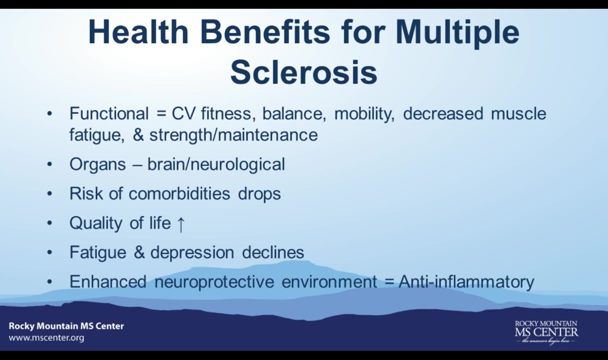 I didn't get into that, I'll be right back. So physical activity has shown to be beneficial to MS and other neural related disorders, And here's where physical activity benefits people with MS the most. And you can think of inactivity as having a negative or opposing effect to the use. 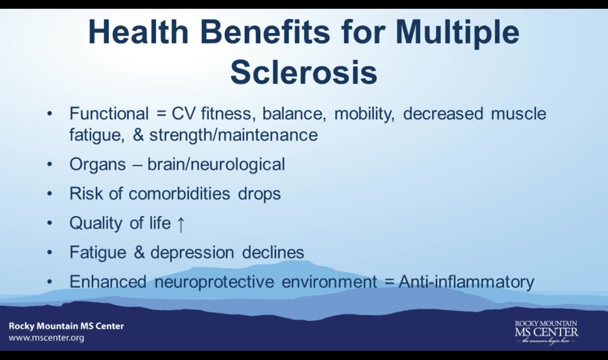 It helps improve or maintain functional ability, leading to better aerobic fitness and increasing or cardio. It helps musculoskeletal strength gains, or at least maintenance of muscle and bone strength. That then feeds into improved balance and mobility, and physical activity can improve muscle fatigue as well. It'll give way to completing daily activities of 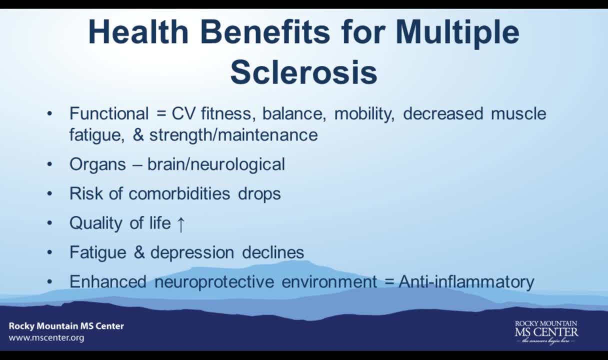 life with greater ease and improving the overall quality of life of people who engage and partake in this activity. Also part of this list is physical activity as it relates to organ function. Organ function as the brain-derived neurotrophic factors BD and F. Essentially, this is a brain function and neurological responses I have listed. 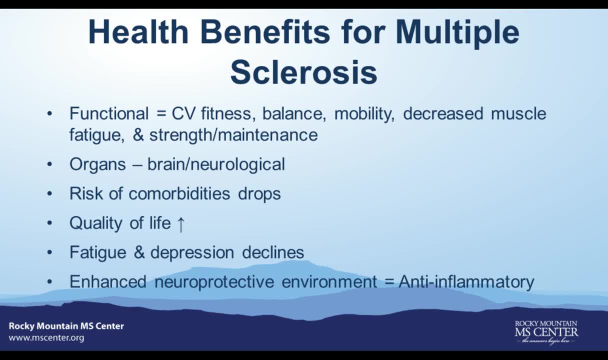 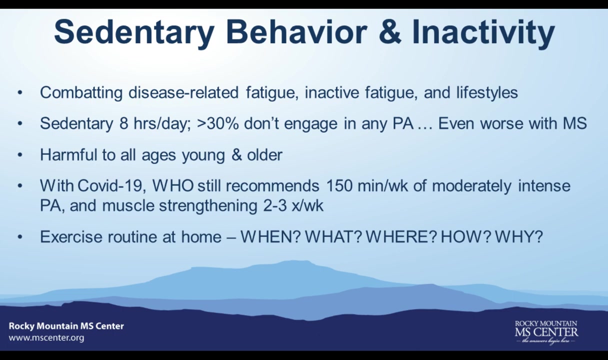 enhanced neuroprotective environments from physical activity, which thus refers to protecting against nerve injury and brain injury. A common factor to sedentary behavior and inactivity with patients who have MS is fatigue, and there's a vicious cycle of inactivity raising fatigue levels even more Equally. 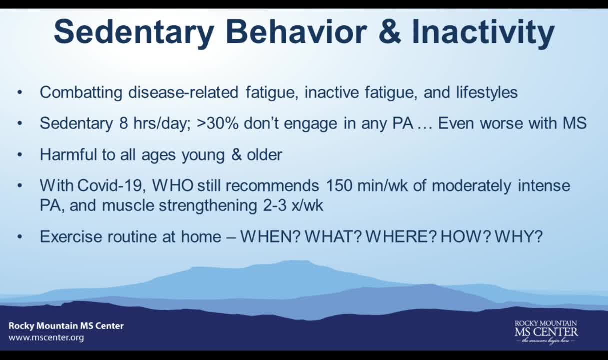 harmful is the nature of sedentary lifestyles to which many people are forced into or inadvertently find themselves in. Additionally, you can find yourself buried in a cycle of inactivity and fatigue, struggling to get out. The other statistic in the second line there is that more than 30% of US adults just don't. 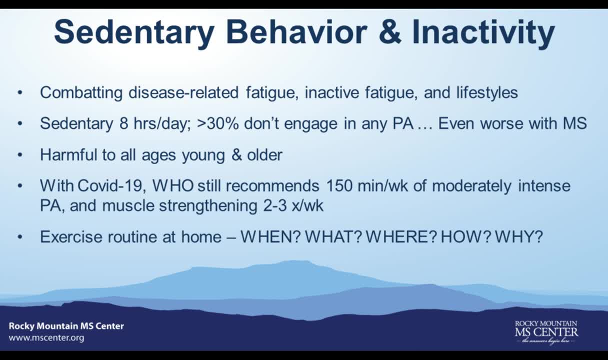 engage in any physical activity in this period. That's the one that hurts my heart. Also worth noting: if you're thinking you're too young for this to be a real concern, you should keep in mind that inactivity is just as prevalent in younger adults and just as equally. 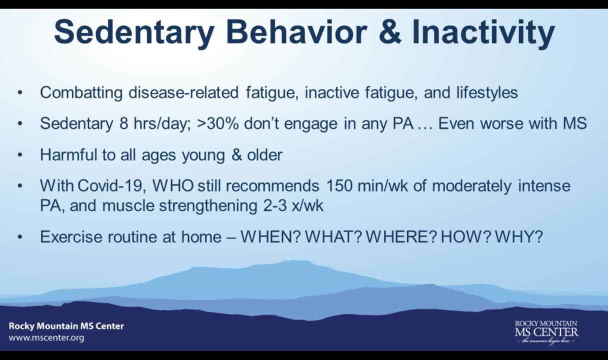 harmful. Studies have shown significant muscle atrophy, which is loss or wasting of muscles, and that being reported after only 14 days of reduced activity in both young and older adults. The World Health Organization, too, has still recommended the same amount of physical activity. 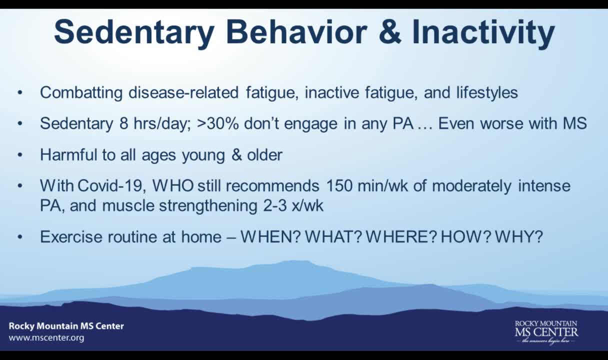 during day or safer-at-home orders of sedentary lifestyles. So I'm going to go back to that, Thank you. Okay, good to see you everyone. Thanks for joining me. I was just going to add that I haven't much information on the. 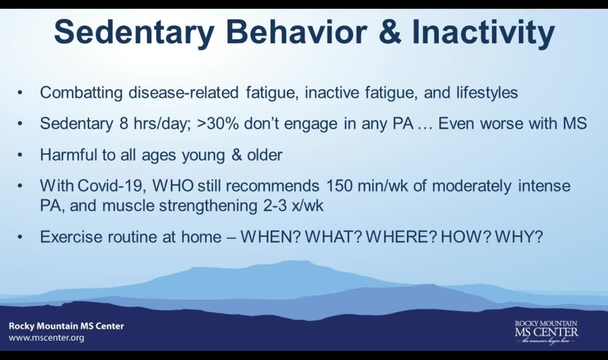 YouTubeiki page they always have. It's listed there About 30 minutes of activity five times per day, or sorry, five days per week to get you up to 150 minutes per week. But if you're at home, then when is it best to work out? 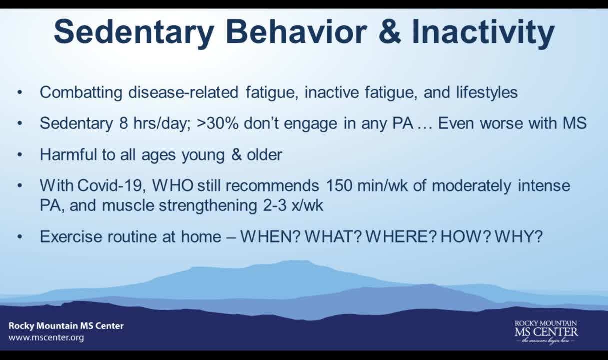 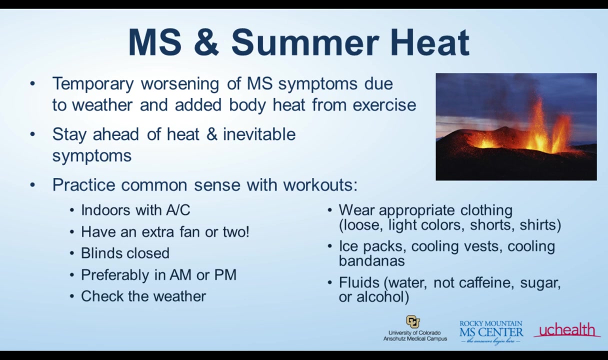 What should or can you do from home Harry Potter's storage closet. you might also be asking: how should you be working out, and well, the why of it. well, hopefully you have been listening and you have a nice idea why it's important to be active, so important one here, when 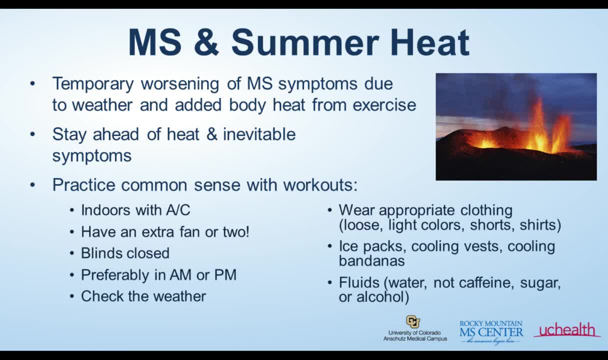 you work in the summertime. as anyone with MS or those who work with clients who have MS knows, it's like all of your, your work, when you're in the heat and all of a sudden it hits you, it's like all your worst symptoms come out at once. 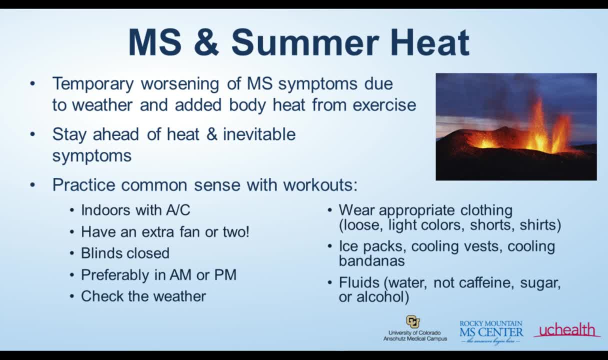 and it could be completely uncontrollable. we have a client at KDEP who we took as part of the trip. we took him frisbee golfing or golfing, and the second time we took him he was a little bit more active and he was kind of. 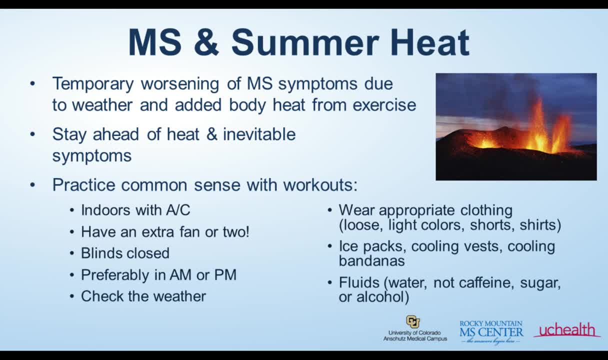 this client. he loves attention and that day he had a one-on-one with the instructor and they played the nine hole course and the instructor was his captive audience, something he also loves. he loves stories. this individual, he's a fairly active. he's fairly active and follows sports and typically he loves. 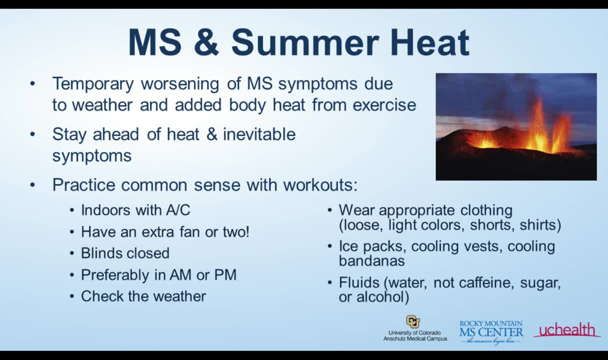 being outside typically, but this hot day and the Sun led to a physical meltdown afterwards. take some points. other things: he loves his food so after falsing in the Sun for solid hours and finishing to take a break, he couldn't even hold his sandwich, let alone bring it to his mouth to eat it, and he's fallen and he would have. 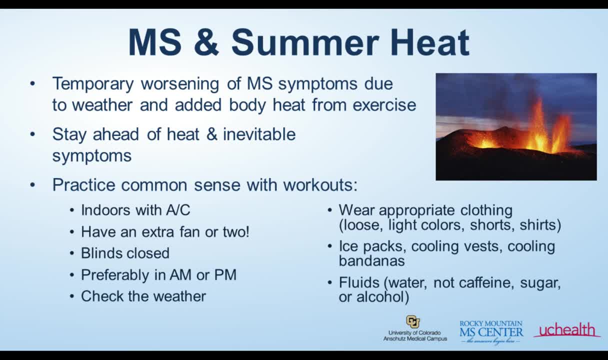 fallen out of his chair if not for a seat belt and us basically supporting them and holding them trying to hold up his torso in place. he eventually recovered eyes on, but it took both of them. that that happened early on in my first year and scares us living daylights out of me. so the lesson is to predict, to predict the 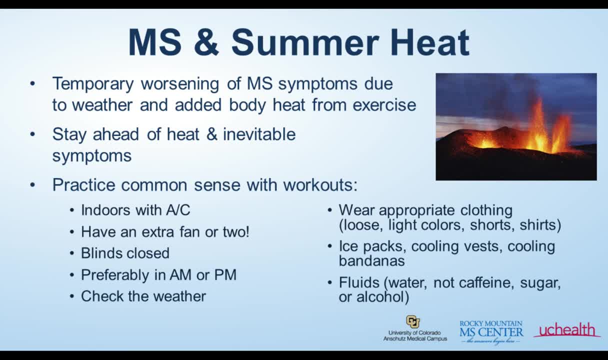 worst, especially during summertime. right now, stays of the heat and inevitable symptoms also practice common sense with physical activity and workouts. the indoors and the nice AC. I have multiple fans and in at our fitness center I recommend at least one. keep your blinds closed. workout in the morning or evening. 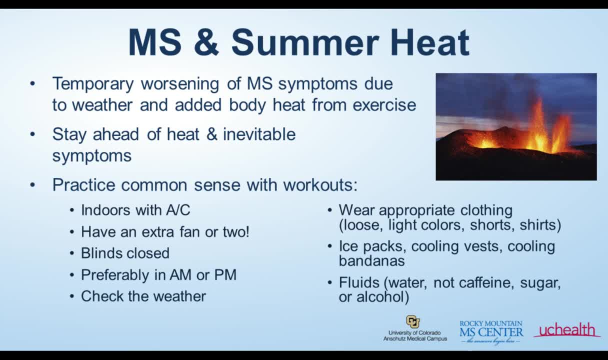 time and check the weather. I I hate small talk on weather and everyone seems to think they're an expert. talking about whether that's also, I hate it, but when it comes to my working out, you betcha, I'm taking a quick peek at a weather app. 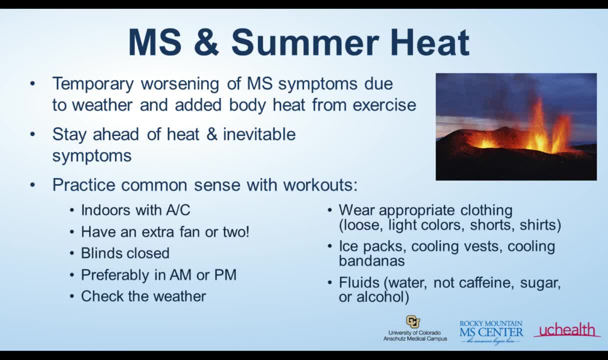 to make sure I'm going out at a appropriate time. also, wear appropriate clothing and invest in all the cooling supplies. ice pack, that's doing that. Danos have the have the right tool for the job, essentially, and drink sea water, the appropriate fluids, avoid caffeine and sugar. I don't know anyone who can. 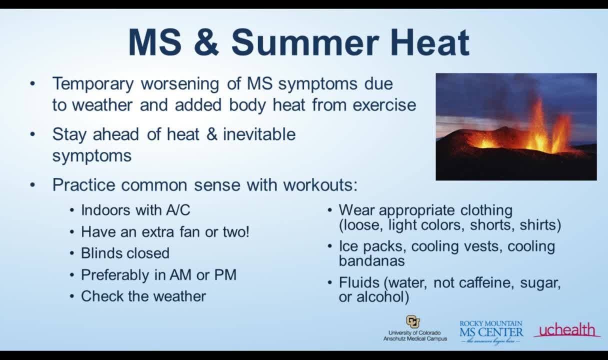 exercise effectively after drinking alcohol? I certainly can't. I tried and in general with fatigue, do a check-in on how much work you are putting in. you know your own endurance. the activity causes 10 out of 10. where you were so short of breath that you couldn't talk, did you experience some pain or numbness? 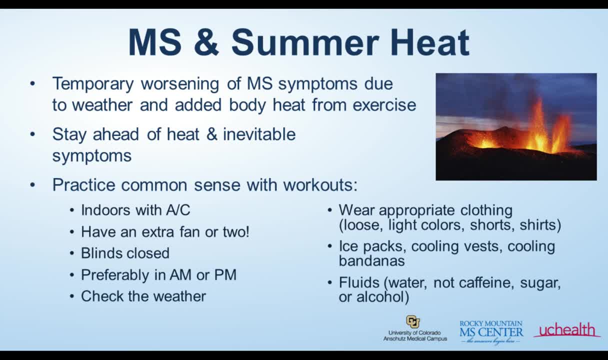 which is these are. this is happening to you and that's the case. I want you to stop that activity and find something better, because you should only ever feel tired and and a bit more. these cases are all 10 out of 10, and this is perhaps too. 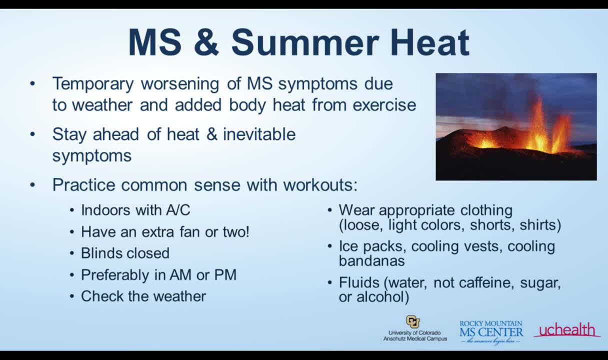 intense of an activity. if you should dial it back to a more moderate level and obviously if you're, they're not doing this. but in the heat, get out of the heat. I don't know why you're working out in the, you know even probably over 75 degrees heat in the first place. also ask: were you? 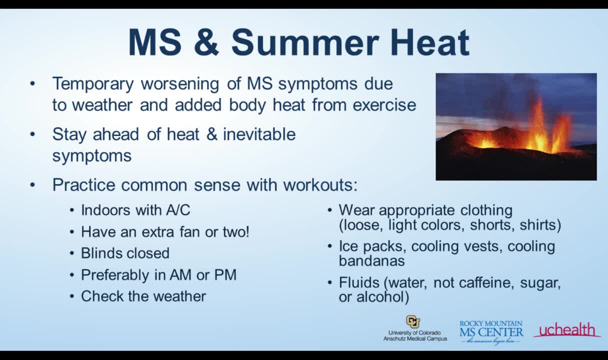 tired but could bounce back to a normal level where you completed your everyday tasks afterwards within an hour of stopping a physical activity, because this is where you should be at. you should be able to continue on with your, your day, without basically a little bit of physical activity just ruining everything for you. 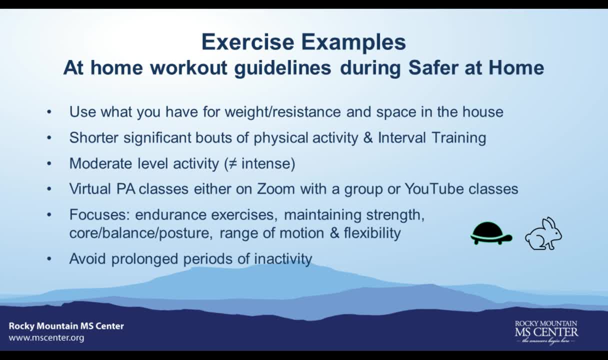 um. so here's some quick guidelines for your at-home workouts. before starting exercise, you should ask yourself what kinds are best for me. what adaptations must I make for it to work? what are the benefits? will I reach my goal and always adapt your routine to set your current fitness level or lifestyle? use what you. 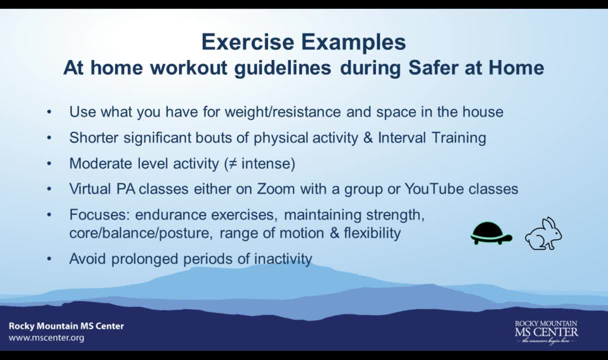 have for weight and resistance and do it within the space, fortunate confines of your house and working without an excuse to do it within the space or to the confines of your house or to the home. and do it within the space or to the confines of your house or to the home. 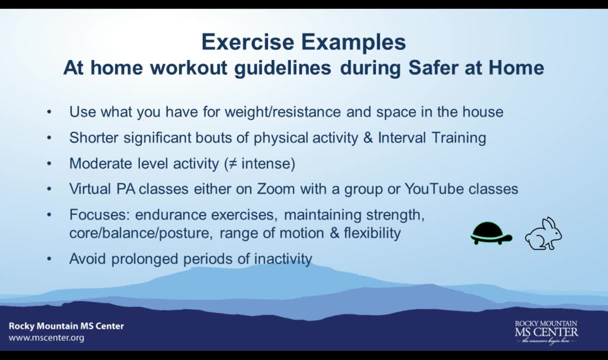 In terms of weights, I had to buy myself some new bands to work out some foam at the gate, as the government shut down and everything, and they're pretty reasonably priced. honestly, It was a good buy. Other weights, though, that you can use, and don't be ashamed of this, because everyone's. 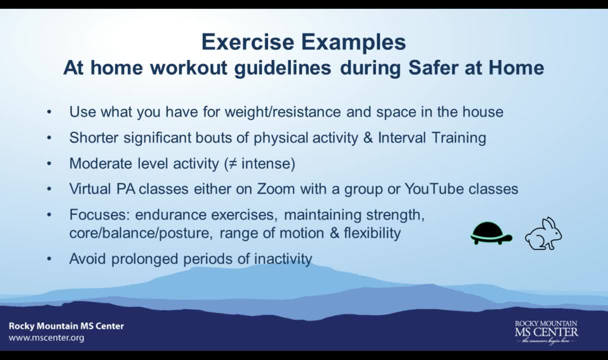 in the same boat right now are non-spillable: jars, cans, detergents, books, liquor- I mean soda bottles- whatever is non-breakable or won't cause a messy bath time. Obviously, if you have hand weights, med balls, actual benches or machines, then you're ahead. 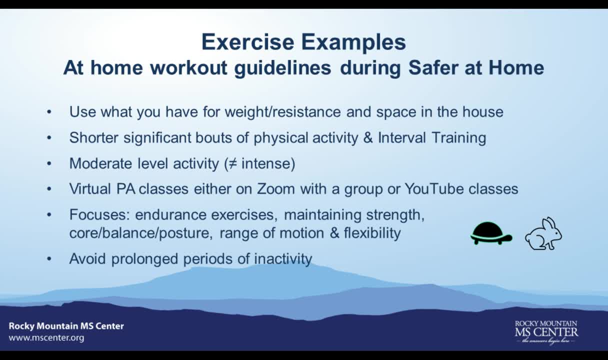 of the curve to use those And with spacing in my bedroom, turned study, turned workout room, turned zoo meeting room, I've found I can still get a lot done from a chair and just finding space for my six-foot wingspan Walking. I'll give you a single step exercise in a minute or two on the next slide. but 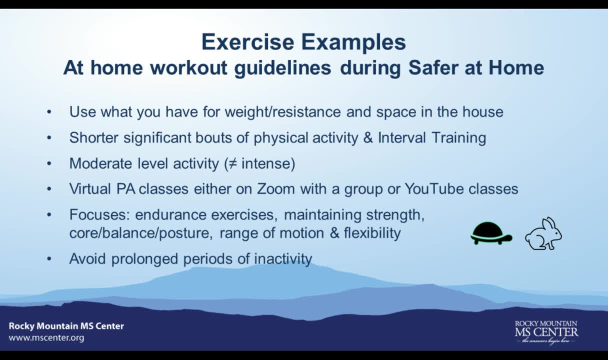 you've seen clients walking back and forth on the sidewalk in front of their homes or indoors in 20- to 30-foot hallways. Every little bit of physical activity is incredibly significant right now in working with what you have. So use your space that you do have and don't discount any ghetto solution. 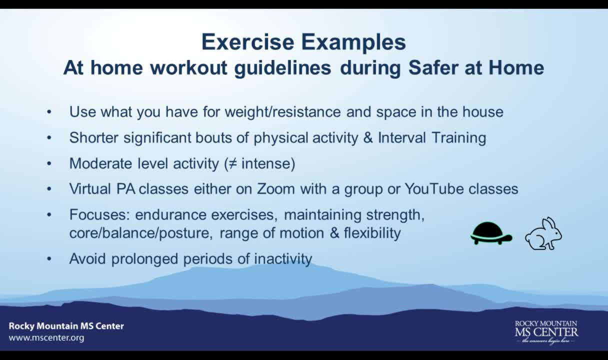 The recommendations from research and presentations, Especially the one that was recent during the MS Educational Summit, called for shorter, significant bouts of physical activity for MS patients. I would apply it as well to anyone with a neurological disorder. Use short, significant bouts of physical activity like a form of interval training- again significant, 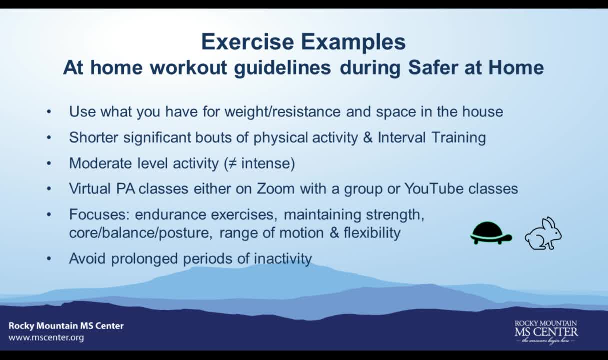 activity, Meaning that you are extending. Okay, So you can use a lot of energy in the form of breathing while you feel comfortably but more heavily, and you can feel your muscles doing the work. Now all you need to do is moderate intensity, as in if you were painting a fence: walking 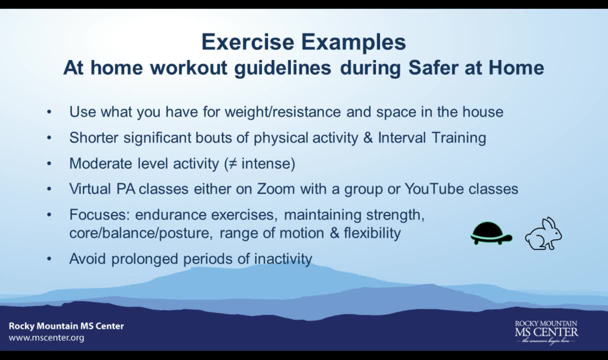 with purpose or pushing and pulling around a vacuum. This moderate intensity varies from person to person, of course, and it is advised to not do intense levels of physical activity. That's the Torch. Okay, I don't know if you can see it on my side. maybe you can see it on your side. 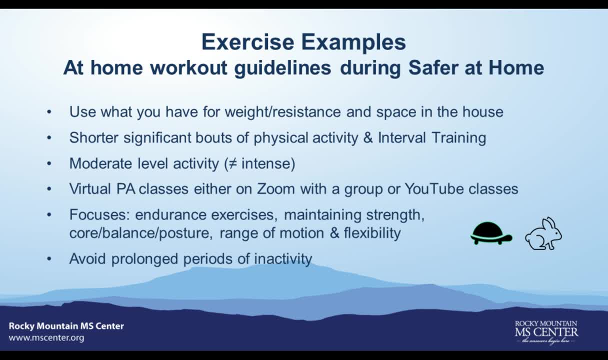 So, yeah, Think of the tortoise and the hare analogy there. You're not doing yourself any favors by trying to go all out, And that's where other symptoms can flare up dramatically, or the elevated fatigue and soreness will cataract your results from doing intense levels of exercise. 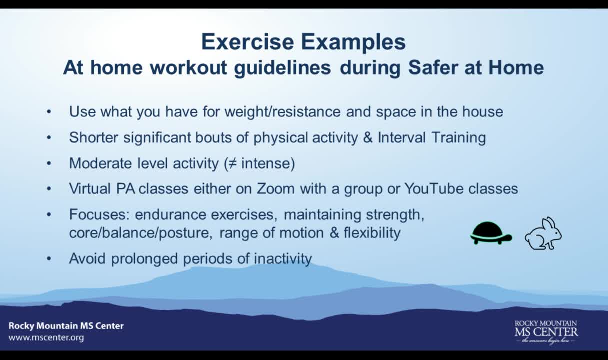 Moderation here. If, joining in on Zoom classes offered online or perhaps through Facebook, you can also find this moderate intensity, I would lean towards yoga, tai chi and basic seated exercise classes. There's a slide on there for you Or invite on there as in through YouTube and just different sources online. 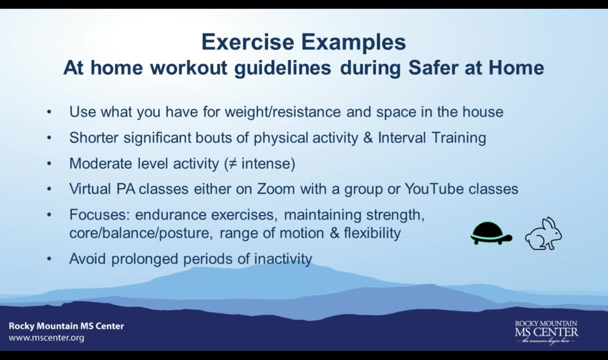 I'll actually mention as well here in a bit. Or you can invite friends online to partake in your own workout classes, once again through Zoom, Skype, Hangouts, Teams. All right, That's how you do it, FaceTime, whatever. 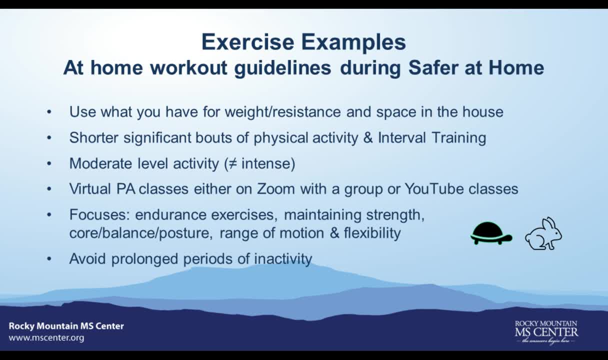 And what I know I like to do when I've worked out with friends is just to trade off with your workout buddies each time on who's bringing in the workout for that session, or follow a workout video together, which I know. there are ways to share your screen during Zoom. 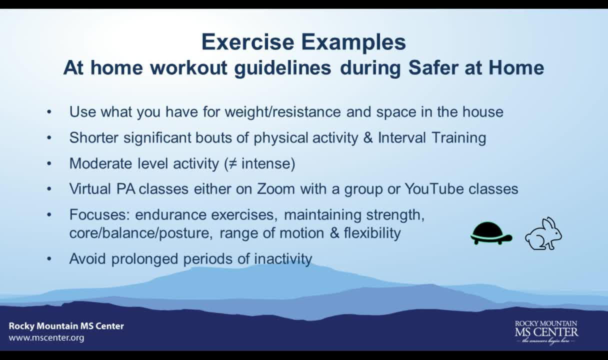 calls. It's not the perfect system, but it's what we got to work with right now. So there is a way to share workout videos and do them together, And it doesn't have to be long, just a half hour or less even. Another thing to note quickly is that the dose or types of 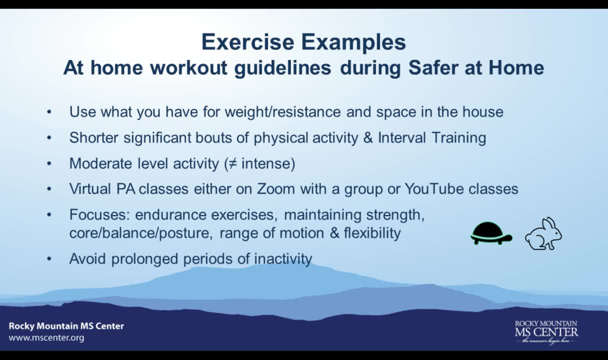 physical activity and durations are going to be prescribed on a case-by-case basis or depending on the individual, So it's hard to get into that here, talking at you all, not knowing most or all of you. Instead, focus on pushing your heart rate comfortably up for a short duration. 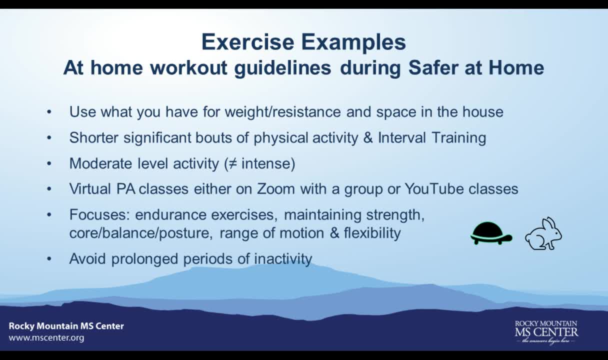 feeling your muscles work, improving your core balance, posture and increasing your range of motion and flexibility. Do some reps, Take a break. Don't focus so much on an acceptable number of reps or seconds. Just watch the clock or use a stopwatch: a start stopwatch. Start small and 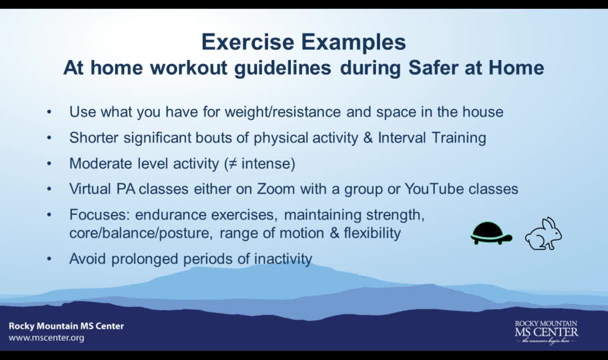 know that any physical activity you do is going to help you dramatically, especially now. Lastly, become physically active. Reduce sedentary behavior by avoiding long periods of nothing but physical activity If you're not physically active. reduce sedentary behavior by avoiding long. 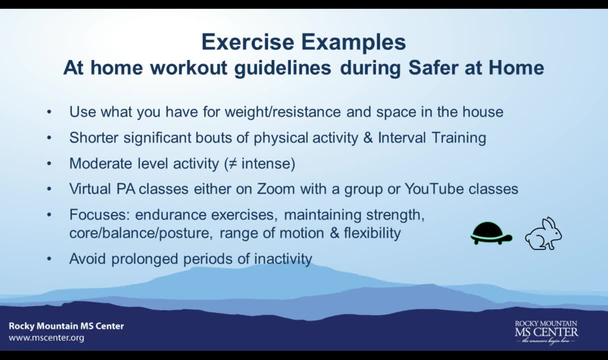 sitting or binge watching a Netflix show for hours on end. Break this up with even quick five-minute activity sessions, Utilize online classes, exercise classes and use smartphone applications and wearable activity trackers to keep track of movement and find some more motivation here. And in case you are wondering, yes, my coworkers and I have found that a step. 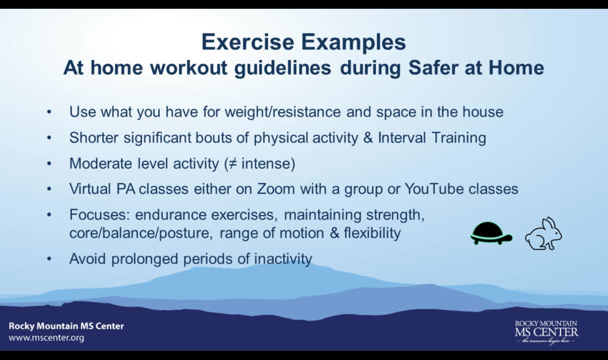 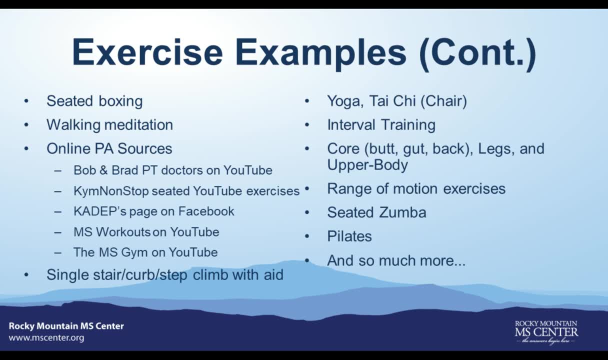 counter and activity tracker will measure upper body movements too. Here is an actual list of exercises and examples to do and to use those guidelines we just set out. In all actuality, you can do a YouTube or Google search and find just about any videos. 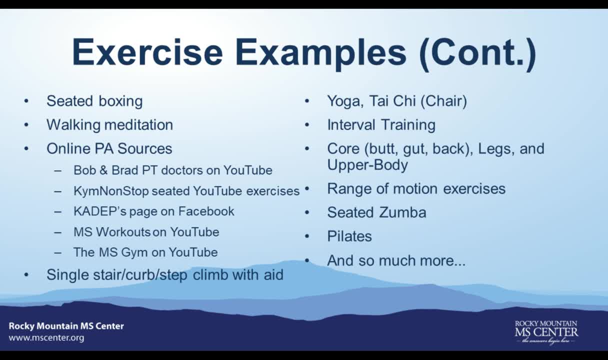 pictures, demos or whatever type of exercise you want to try now. Just be smart with it, Such as I typed in: show me any seated upper body exercises And I suddenly had a wide array of options in front of me, Some other online sources I like I have typed out there. Take a look and get creative with your. 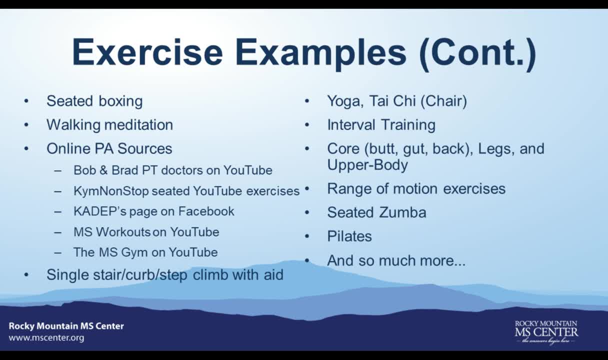 own workouts. As long as you're kind of following the guidelines we're setting up here, you should be safe, And that is at the forefront when you are working out. Just be safe with it, especially at home. One other pro tip I'll point out is if you also focus to work on your form and keeping your 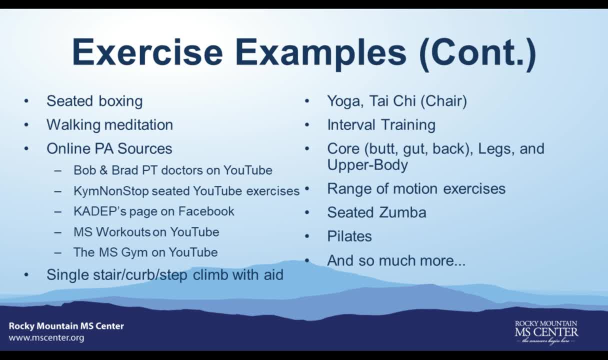 abs or tummy tight, as well as your posture: upright and without back support, maybe leaning a little bit away from your back support to engage your core. you're working on multiple muscles and doing more work, therefore getting more out of the workout and less time. 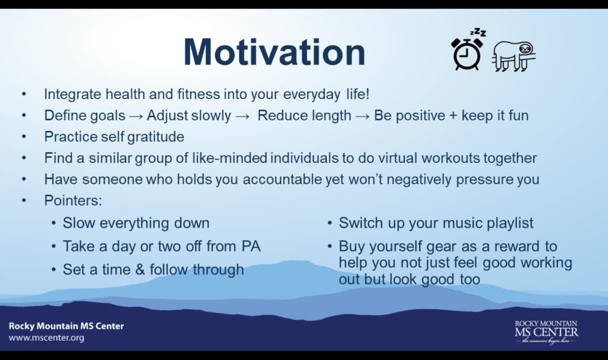 The last, one of the last few things here, with where we're at now in the world. motivation, speed, activity and how to get your body active can be especially hard to find, if it wasn't already hard before all of this. Make your health part of your daily routine and incorporate it fully into your 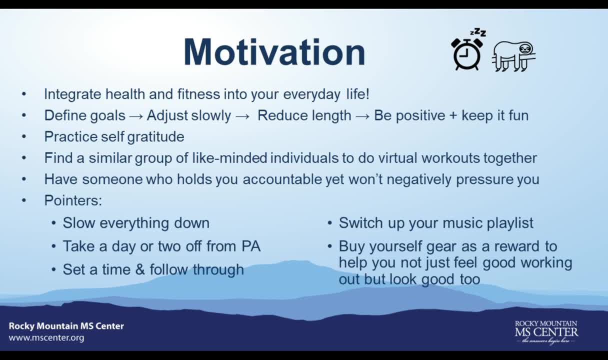 lifestyle. Define your goals by figuring out the ideal outcomes, how you can get there, roadblocks that might come up, pros and cons- and get it all down on paper to look back on and reference. Adjust slowly and progressively, especially when incorporating new fitness goals. 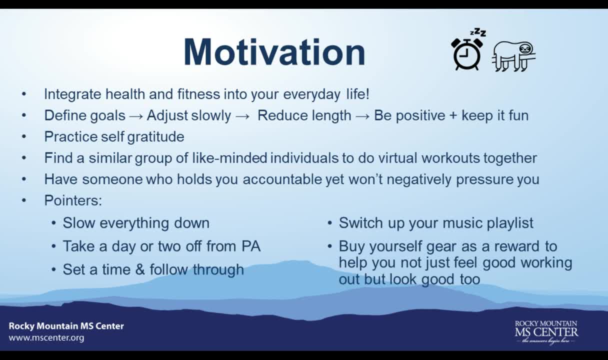 You're also going to want to take advantage of the strength of your workout to make it less intimidating and to abide by guidelines that we laid out again on exercising and fitness activity. Studies show that saying positive things, practicing gratitude and self-care helps improve. 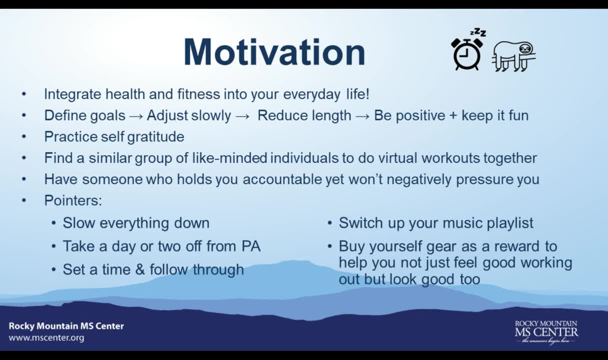 your body image and self-esteem. I in fact read a book recently called How to Un-F Your Brain, although she didn't edit herself in her title. it's by Dr Faith G Harper and it prescribes in one part routinely saying positive things to yourself- And I'm a positive. 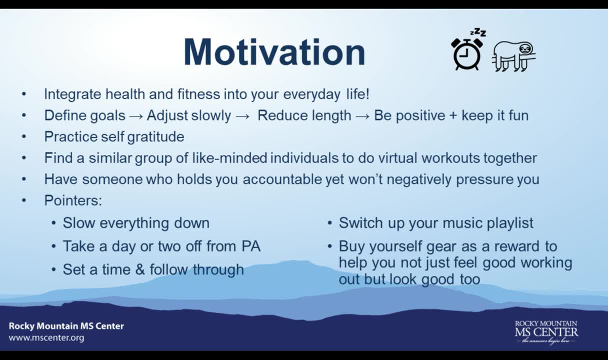 guy around other people, but I realized I wasn't being that way to myself. most times when I was alone I cut myself down and think of all the things I should have done differently, So instead have encouraging mental dialogue. Having that has been huge for me and I certainly recommend it. 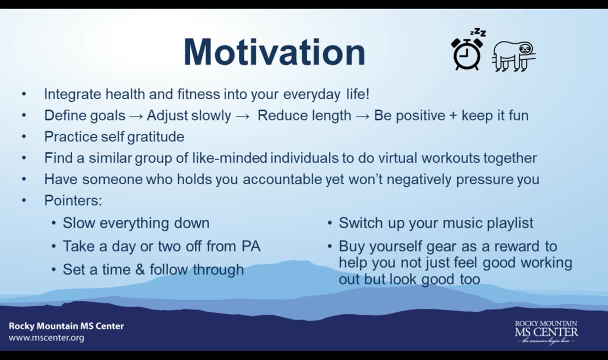 In addition to being positive, keep it fun. whatever you're doing, Don't do an exercising exercise. There are so many other options out there and things for you to try out. We mentioned in a previous slide working out with groups, virtually like I said. 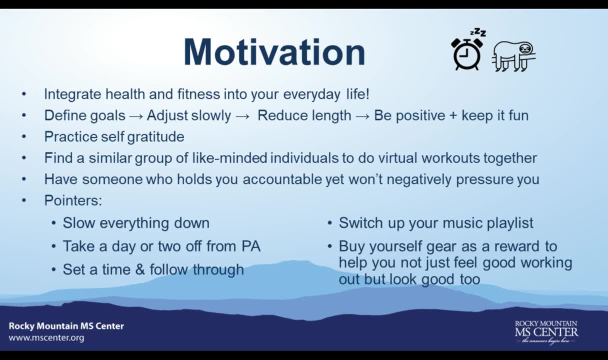 quite a few times, actually, This can help, though That's why I said it a few times: Find a group or someone who holds you accountable yet won't negatively pressure you, So this might not be your spouse. In the same way, a lot of people can't work with their spouse at a job. 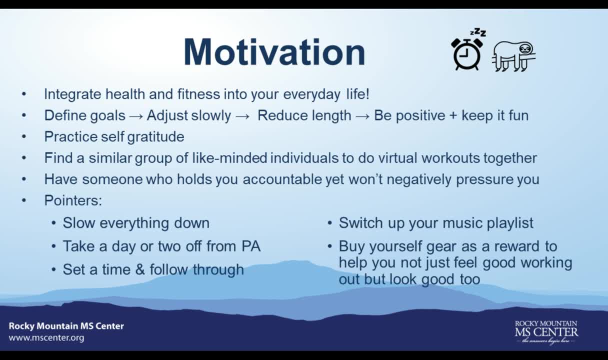 you might not be able to work out with your spouse or see this other either. Find someone on the same level as you. I'm a proponent of meditating. It definitely helps to slow everything down. It's the whole Ferris Bueller line: Life moves pretty fast If you don't stop to look around. 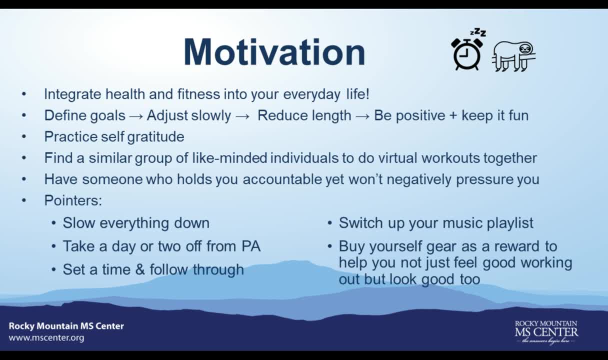 sometimes you can miss it. Figure out what helps you slow down and focus, whether it's meditation or something else. Take a day or two off from physical activity, because A it's recommended by organizations such as the American College of Sports Medicine. 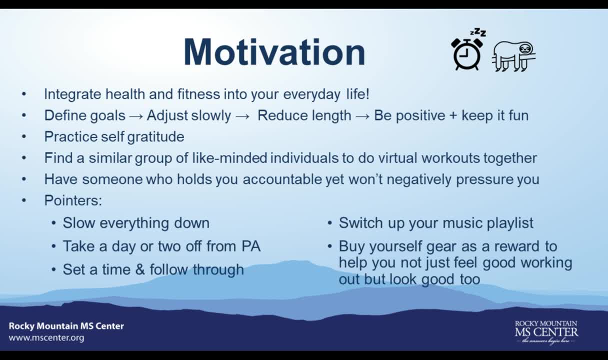 and other high-standing organizations, and B exercise is a life of effort. It'll be there when you get back. You can guarantee it. Set a time, Follow through, but realize if you are just starting out on a healthy routine. 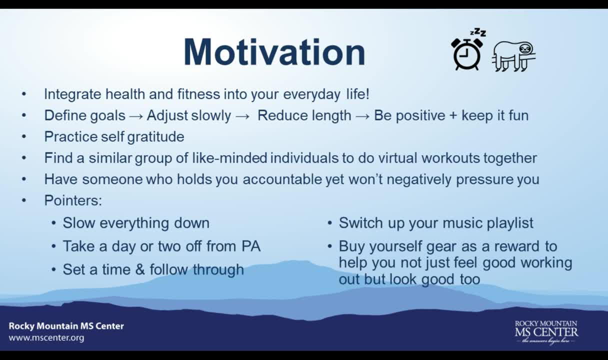 you may need to retake that first set multiple times, But if you keep taking it again and again until it's a habit and you're contained to maintain that routine. I love music. Highly encouraged. We've laughed. Taylor Swift and who's Hannah Montana? Miley Cyrus- all the time in the fitness center. 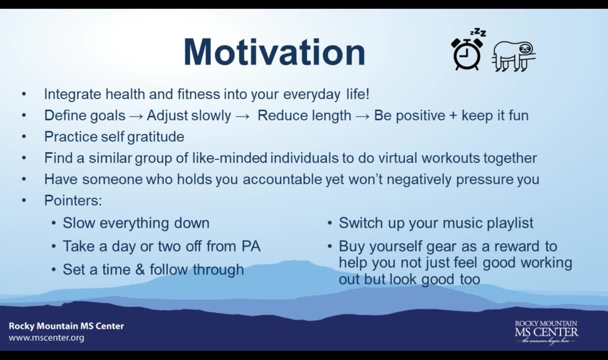 If the clients don't love it. I love it, But either way, put on some music, It'll help motivate you, I feel like, as well as watching and listening to virtual nature walks, This is actually a good way to kind of find different levels of focus and meditation, as 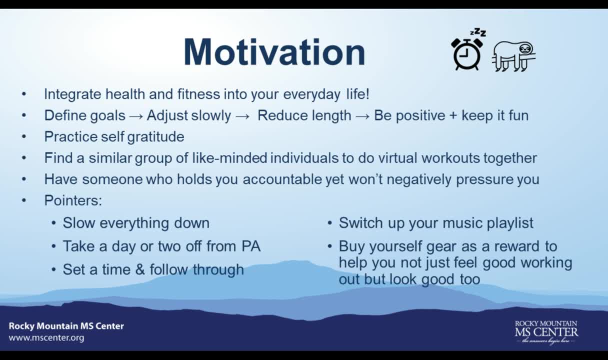 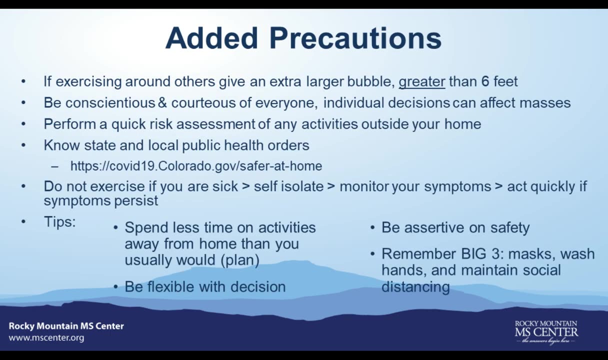 you're working out. There's a study of research talking about getting nature and listening. listening to nature as you physically move, It definitely helps. But last thing, by yourself here, feel good, look good, And then just a PSA, sort of a PSA, extra precautions to use at this time with. 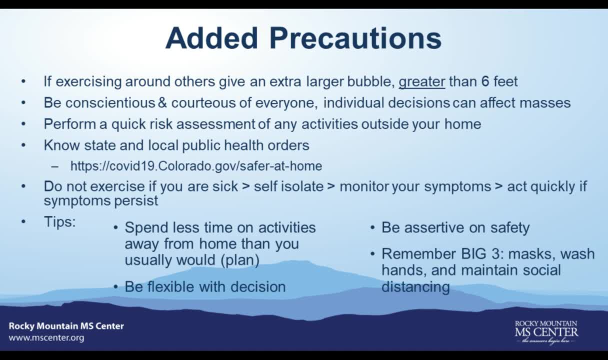 paper and foam boarders. Remember that you'll be breathing harder during activities, so you may need to stay farther apart from others. Ready, I've read, suggest more than over 15 feet actually, while if you're vigorously breathing, and breathing hard as you're working out. I know that's not the easiest thing, but 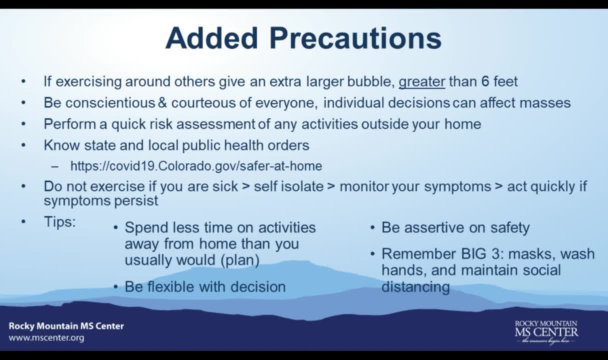 it's more than six feet, So keep that in mind. Be conscientious and courteous of everyone. Individual decisions can affect masses, As in people you live with. be conscientious and courteous of them, Loved ones, who you don't live with but maybe want to visit again soon. Think of 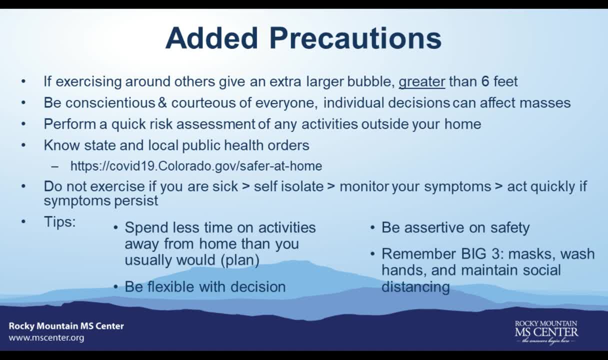 them and be conscientious and courteous to your surrounding community, others around you. You might not see them, but there's elderly people who are immunocompromised and others who are just generally at a higher risk, similar to our MS and neuro population. 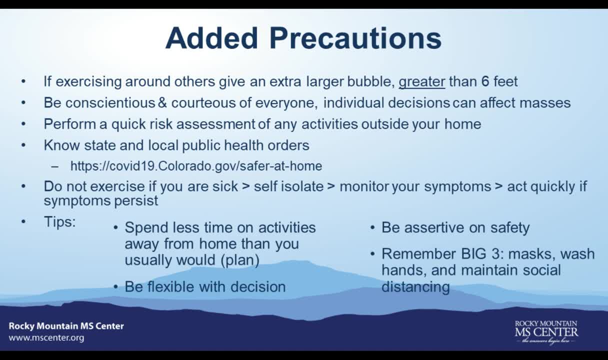 Perform a quick risk assessment of any activities outside your home. How many people are involved? Is it indoors or outdoors? Is the risk to reward ratio actually worth it? Also recognize that if you have any other medical conditions along with multiple sclerosis, what may be low risk for some people may not be low risk for you. 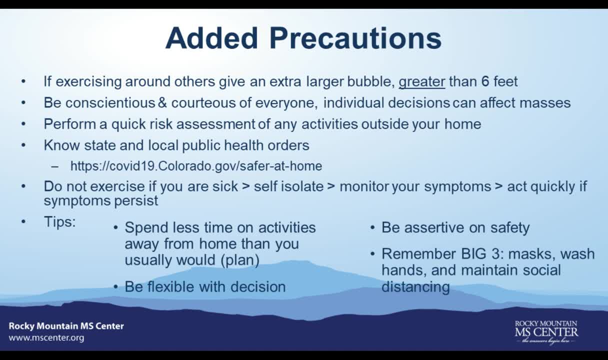 Just because a business or facility opens doesn't mean it's safe for everyone, unfortunately. Take close attention to state and local guidelines from authorities for specific activities. A great source that I mentioned at the beginning and I'll mention it again, is through Coloradogov. 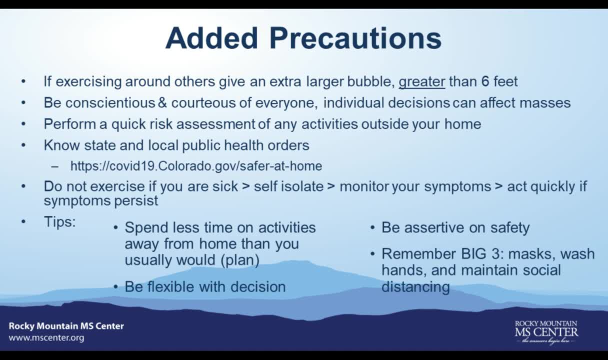 at covid19.coloradogov backslash saferathome website. I looked at it a bit and it's truly helpful. There are tabs on there specific to outdoor recreation and personal recreation on there. even: Do not exercise if you're sick. If that's the case, self-isolate, monitor your. 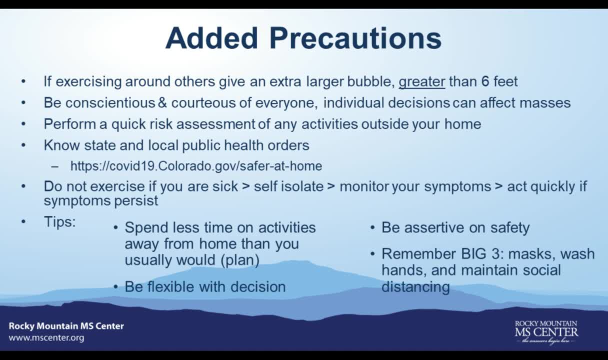 symptoms and act quickly. if the symptoms persist or, especially, it seems like, if they're unusual to you, Be sure to contact whether it's emergency care or a family member that can help you. The tips here are obvious. The one I'll recommend and reach you is to be assertive on your own. 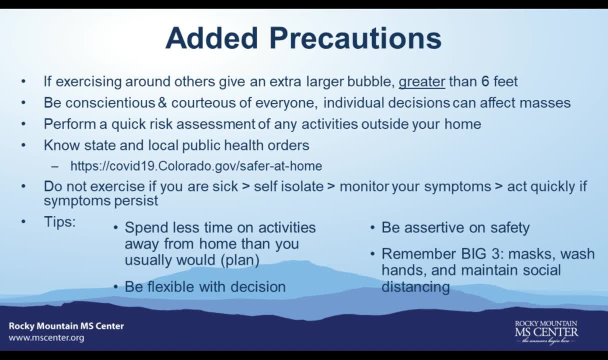 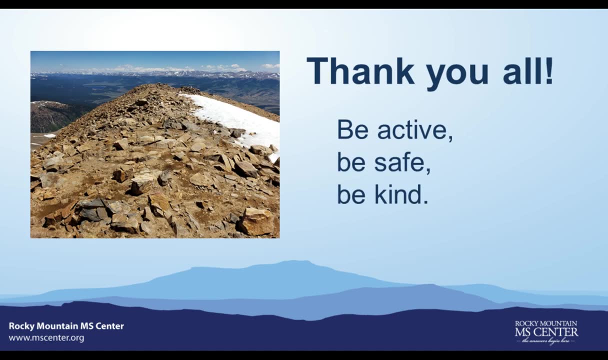 safety and on others. Don't decide to just throw caution into the wind. Wait and listen for health officials and medical doctors to advise you on the best course of action and when it's safe to get back to our lives. So I want to just thank you all and I appreciate you listening to me. 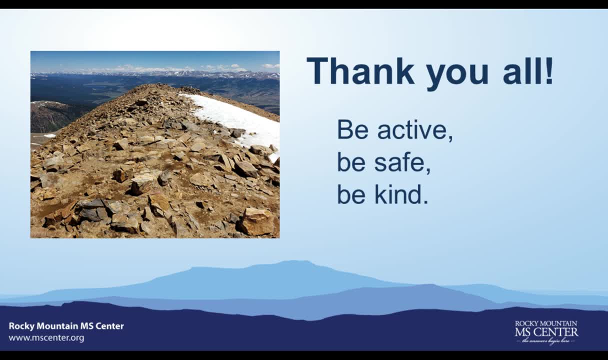 Thank you, Ryan. If you have a question to submit, you can do so now using the chat window on your screen. We are unable to give specific medical advice out during this webinar. If you have questions relating to specific DMTs and your MS care, please discuss these with your. 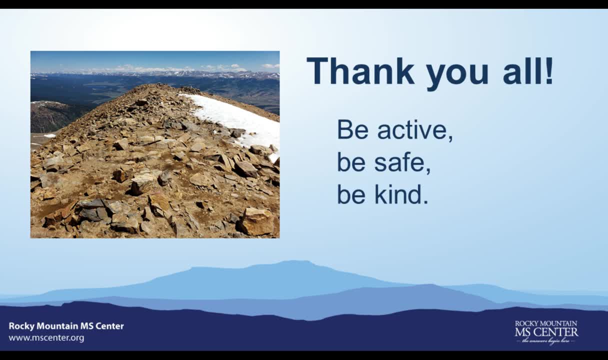 neurologist. And then I also wanted to point out a couple of resources that we have available before I move into the Q&A. If you have any questions, feel free to put them in the Q&A section of the Q&A segment. We do have that COVID-19 education page, which can be found through mscenterorg. 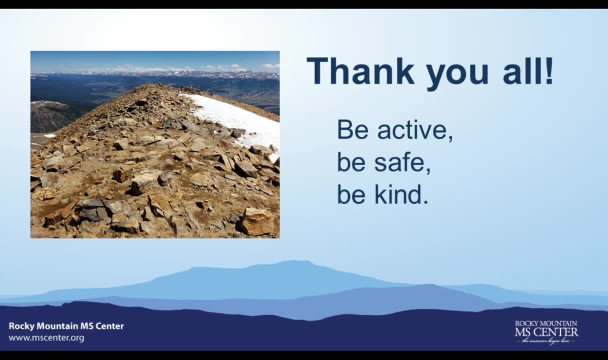 It's got several webinars featuring Dr Alvarez answering MS questions. It's got a document on it called COVID-19: Resources for You and Your Family, which has many links to physical well-being sites, including specialized adaptive YouTube channels, chair workouts. We've got a recorded. 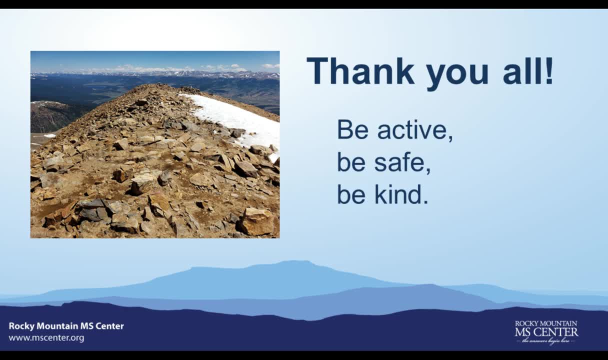 chair workout from one of our staff members. We've got a recorded chair workout from one of our MS specialists, physical therapist Michelle Harrison. If you are looking to figure out how to incorporate fitness into your new daily habits, we have a webinar talking about building new 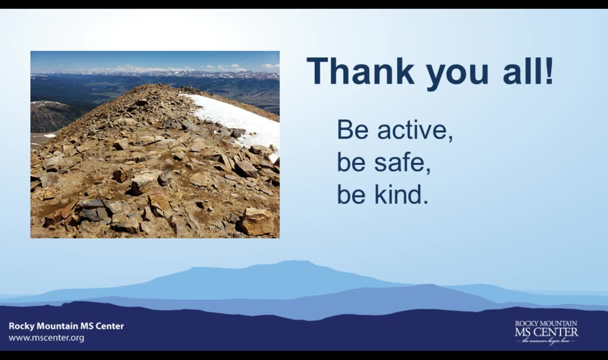 habits also found on mscenterorg. So there's a lot of great information on our website. I'm going to move into the questions now. We had a lot of really great questions submitted ahead of time, so thank you guys for that. Several people asked variations on the questions. 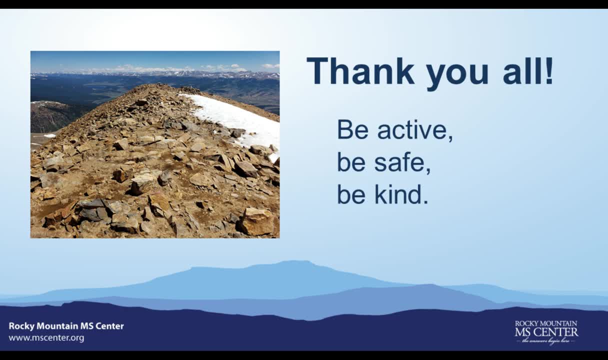 and I wanted to ask what's the best way to build up stamina, particularly when you're fighting fatigue and when you've got MS? What's the best way to build up stamina? Yeah, I felt like we hit on it a bit there and just kind of based off what was presented. 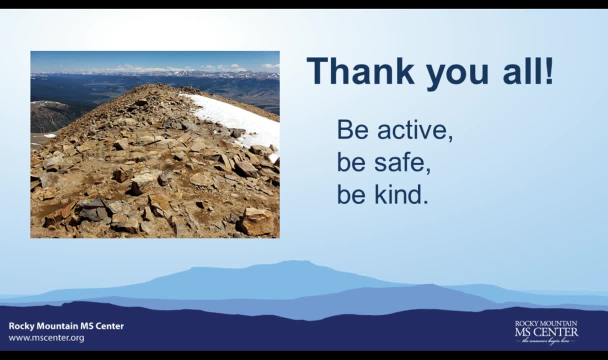 again during the MS educational summit, recommending just building up your endurance and your fatigue levels through like short doubts starting out. you know, even if it's just 30 seconds on, 30 seconds off, you're starting. there You're maybe building up to. 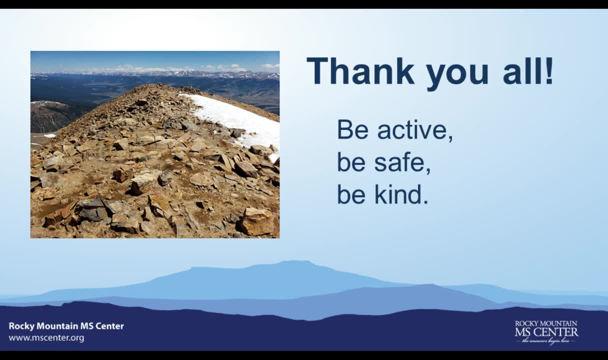 a minute on of like pushing doing your workout and then 30 seconds off and just adding a little bit more each day, or maybe just not until, like each week Working your way up to I was able to workout for just 20 minutes and then just adding a little bit more each day, So I think that's. so cool Serving my patients for today is burnt out. I appreciate it, I appreciate it. I appreciate you, Jim, for having me. I appreciate you for嗎. Please take care, Please take care, Please be well. Thanks, Jim Bye. I appreciate you. I appreciate you, Jim. I appreciate you, Kim, I appreciate you, I appreciate you. 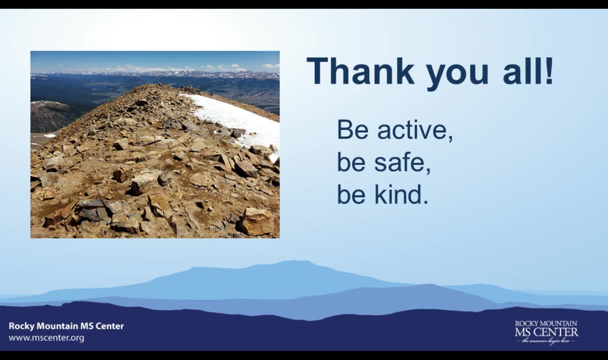 minutes today to then you can maybe go up, go up from there and for you maybe can hit that 30 minutes per day, but start slow. and then of course other other ways to kind of help, help against endurance and fatigue or, you know, doing the cardio exercise. again I stress, starting out slow. you don't need to be doing a. 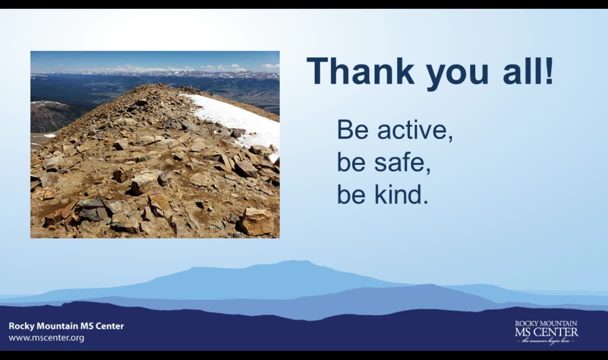 full-on, like 30 an hour, like take, take it in baby steps, honestly, especially if it's not something you've you've done before. so we're talking. you mentioned the guidelines of 150 minutes per week, for I believe that was moderate intensity activity, yes, and then folks were also asking kind of what's the? 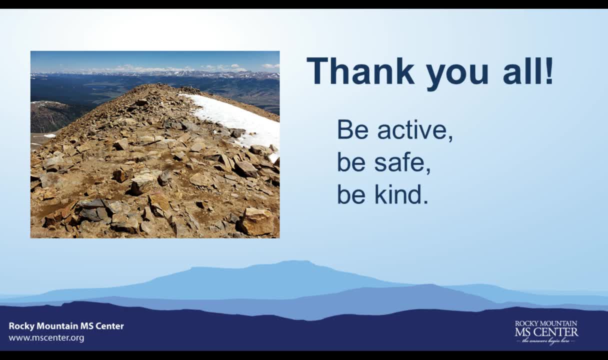 recommendations for combination. if you're going to ask for a combination, if you're going to ask for a combination, if you're going to have in strength training versus aerobic activity. so yeah, the other recommendation there was, to you know, doing strength training two to three times per week. you do want to break them up. one day you might do your endurance. 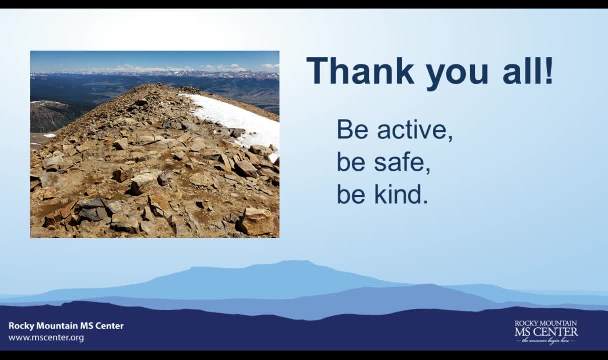 training the next day, doing your strength training. that's definitely the best practice. you don't need to, certainly don't need to double up on on both of them. but yeah, that's my recommendation. so, once again, I'm always going to say, like, start out, start out. well, don't just jump into something that you have never. 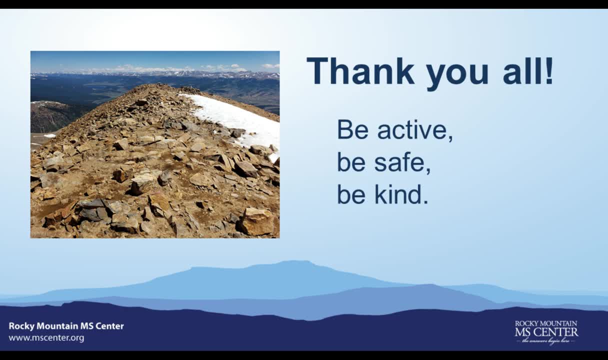 done before and if you it does say 150 minutes, that's for, I guess, an average healthy US adult, I I want to say that I've seen other figures- the next two MS patients- where it says where it maybe cuts back that figure in half. so keep in mind it's really just a number. what you want to focus on more is 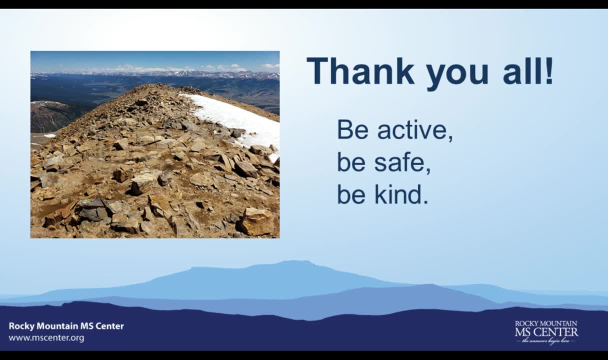 just your, your own individual abilities. I'm going to group a couple of questions all together here because I think they're related. we have questions relating to specific ab exercises, strategies for kind of what kind of exercises will help either prevent a fall or just have you help you have better control, as well as balanced and 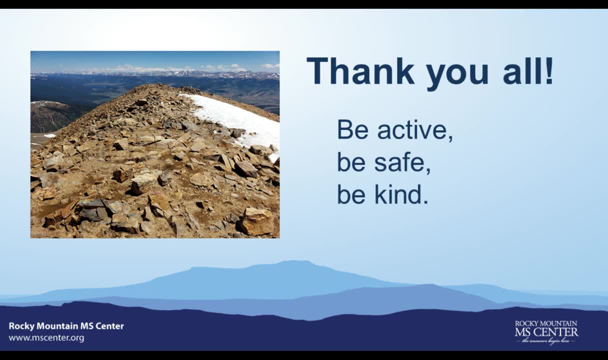 gait, kind of like. those are all similar questions. yeah, so what we're getting at there to help you with with your, your ab workout, your your balance and gate. it's like you might listed one more in their fall fall prevention. you're working on your core, so any ab exercise you're doing on your core jar. 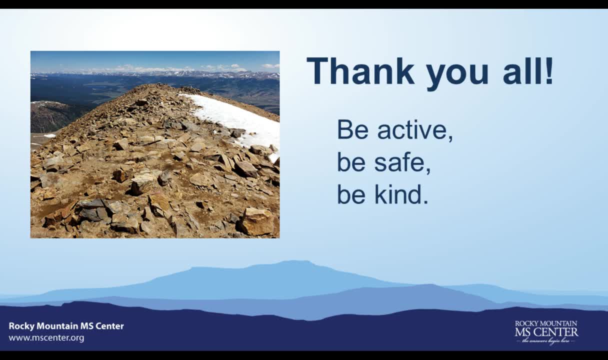 home core routine exercise you could find should be beneficial in kind of helping you with with all the above there there's plenty of seated core routines, as Kelsey mentioned, a lot of resources through our recommend MS Center page from me and some of the other staff on our KDEF page and 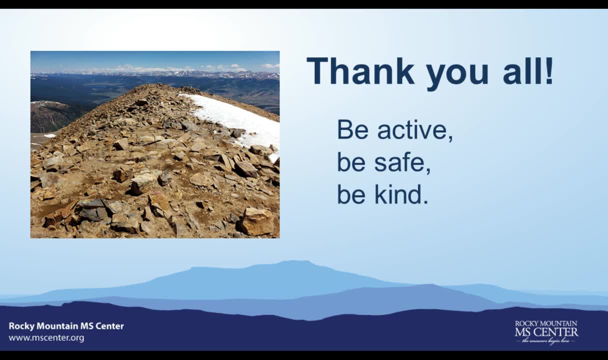 YouTube. but, yeah, you're looking to effectively strengthen your, your core with with that- and I know I kind of hinted on it- just any exercise you do trying to tighten your tummy, stay nice and tall, keep your head up as you're, as you're doing these exercises and as you're doing them as well. try and you. 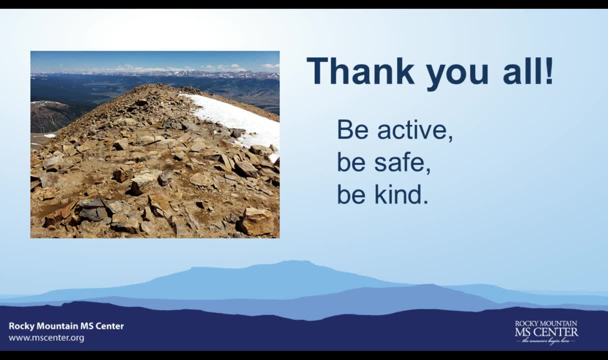 know, be upright and away from your back. support are all going to aid with with support your core workout. and yeah, just taking it, taking it gradually as you go. you know, if you can work your way up to standing, then there's plenty more standing core exercise workouts you can do from there. but taking it, taking it. 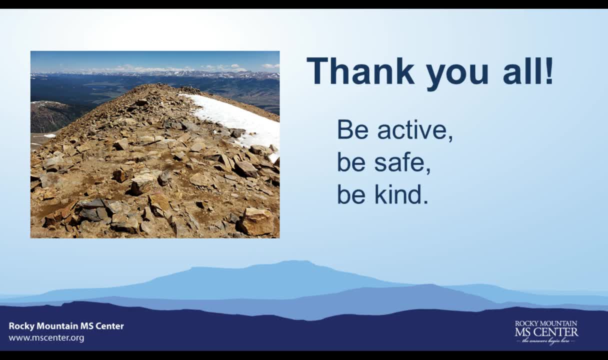 one step at a time. I feel like I'm repeating myself, but that's kind of how it goes with physical therapy and activity. Is standing like using a standing desk for your computer rather than a standing desk than being seated? is that considered exercise or right? so that would be more. 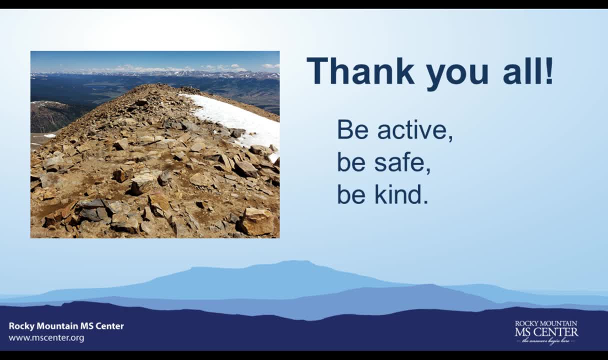 just I'm blanking on the term there's- you can get physical activity just from, yeah, daily, like just standing or basically breathing. so I wouldn't necessarily call it physical activity, it's just kind of like a common activity. but it is beneficial, especially if you're able to work on your balance. and again, like you know, 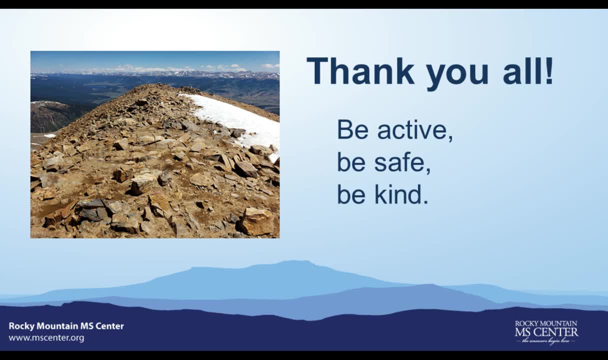 staying tall, at least keeping the correct posture while you're doing it. it is, it does have some significance to your, your physical health. most most definitely the term. I'm trying to think of what, what to call it. I'm blanking on though, unfortunately, but it is. it is beneficial indeed, it's helpful, it just 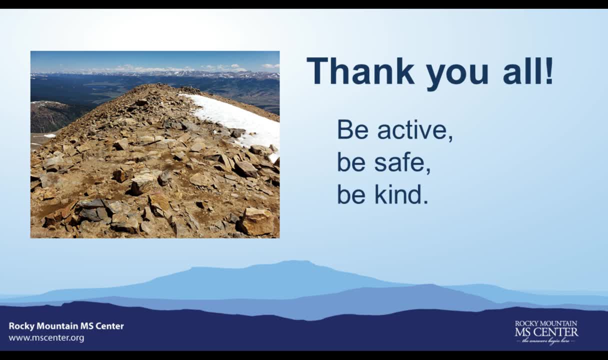 doesn't contribute to those. that 150 minutes or whatever you're shooting for. yeah, it's dumb. that's that's why I'm kind of thinking of delayed. oh no, that's something different. I take it back. so, sorry guys, do you have any favorite chair aerobic exercises or maybe YouTube channels that? 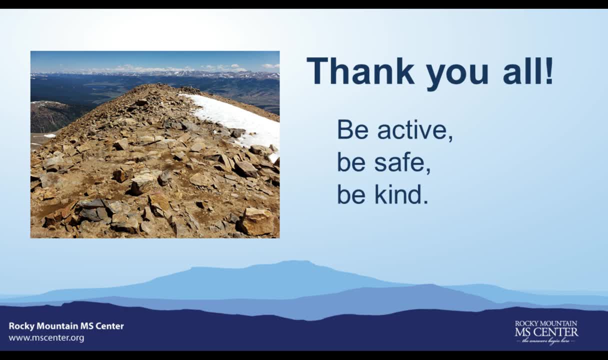 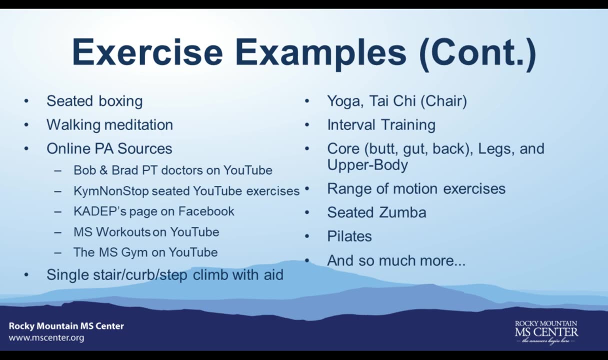 you want to specifically recommend for chair seated aerobic workouts? yeah, the uh there's. there's a couple that I guess I just kind of referenced there. um, let me see if I can slide this real quick. I know I like the uh, the Bob and Brad. they're PT doctors on YouTube, they're. 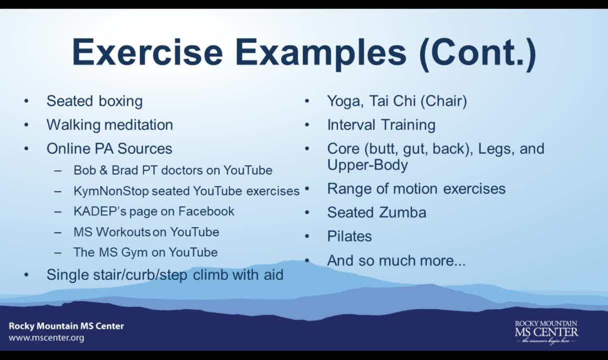 really dorky. I think they're from Wisconsin, but they have great quick little 10 minute videos that hit on a bunch of different things, especially, you know, ailments and and things for MS patients that they can work on. another one that I kind of like- I think she's a little bit more intense- 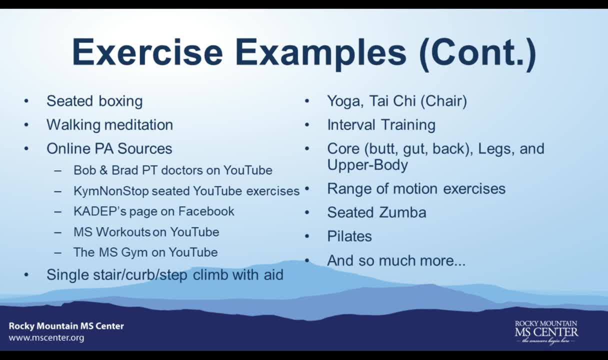 she, oddly enough, has some some good seated exercises on YouTube. it's Kim non-stop. that's K Y M non-stop. like I said, she's a little intense but I I kind of like it. it's a little more um, on the go and moving and and not too too slow, um, those are easy workouts as well as again. 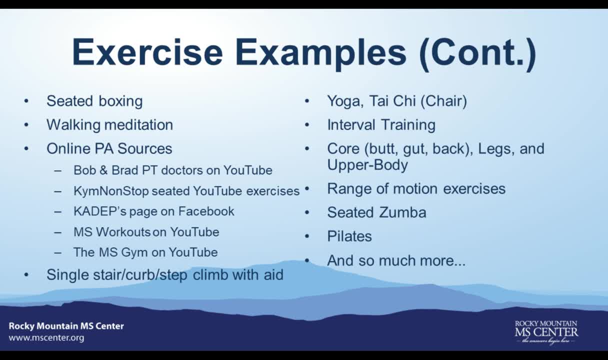 recommended message. page of the few. uh, the other guy, he's a little little bit dorky and he is a little it's a little bit darky for me, but he knows his stuff is the MS Gym and that's it's really. 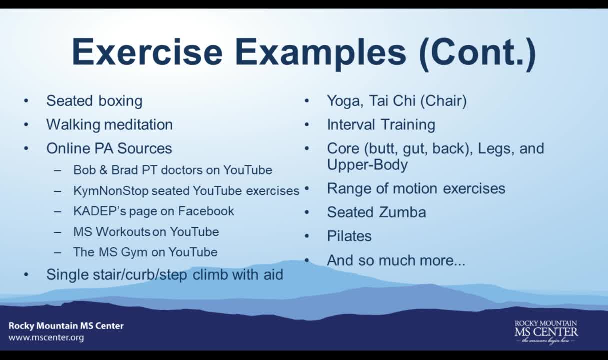 basic, the way he wrote it out, just the MS Gym that's also on YouTube and he specifically has MS, so he's able to truly relate to clients and anyone that's able to watch his videos. And then, do you also have any exercise recommendations? 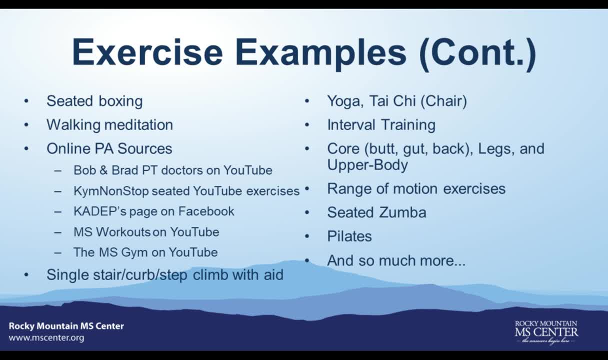 for someone who is confined to their bed. Yeah, the kind of nice part one thing like with my clients is they're basically confined to the chair, but there's so many more exercises and things you can actually do from you know, lying down, or or we I, or if you're working out on a, on a mat, mat exercises. 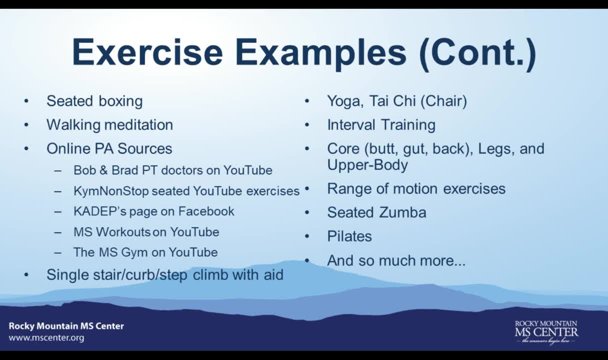 and what's coming to mind is definitely: keep on with your. your a good amount of exercise and I think that's a good thing to do. You can still do a bunch of stretching from you know the confinement of your bed. 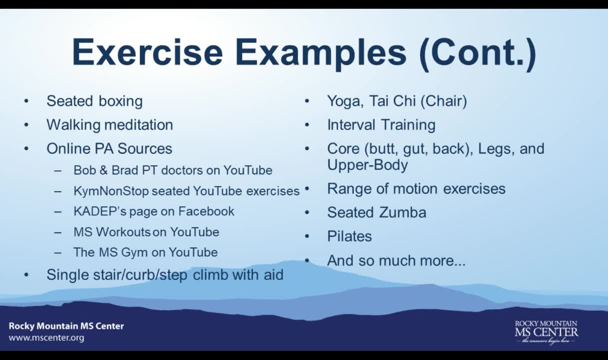 you're, you're laying down, you can. you can do some of the stuff you might do from a regular bench and you can. you can still have, you know, whether it's true hand weights or if you're using at-home like soup cans and stuff. you can still have some weights. 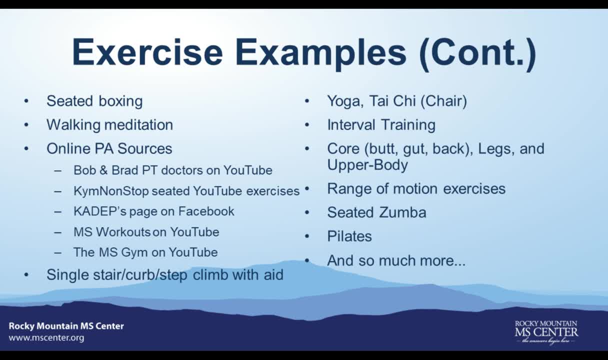 you're doing a, you're doing your bench press, your your flies, doing a few different things, but but definitely getting in your, your stretch routine on the daily and finding, finding some different exercises, whether it's again from like lying down on a bench or 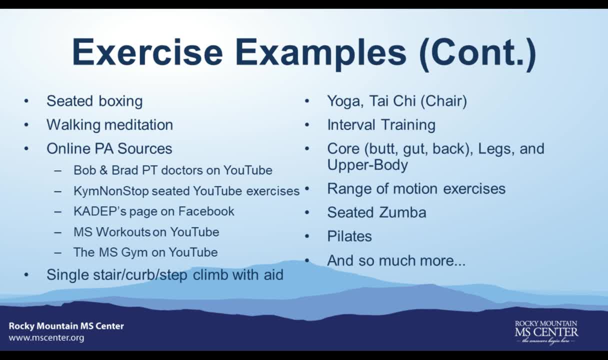 you're in a good spot to be able to do a core workout routine just from from like maybe a fitness mat is what you might. might need to call it or consider it if you're looking up specific exercises to do, but continuing to still stay active. 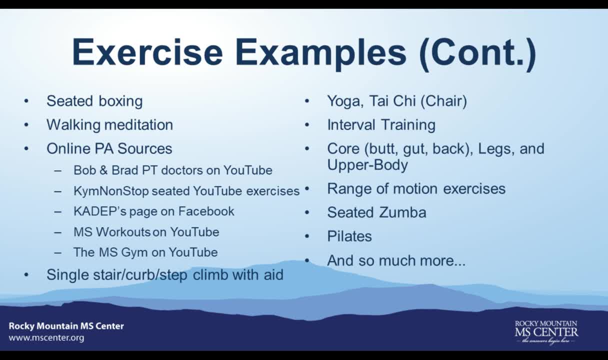 and you can actually still be doing it from from a bed, even if it's if you're taking up your, your legs and your arms like a baby and kind of doing like a, like a stationary bike, only laying down plenty of stuff you can be doing and just be sure to still be active in that regard. 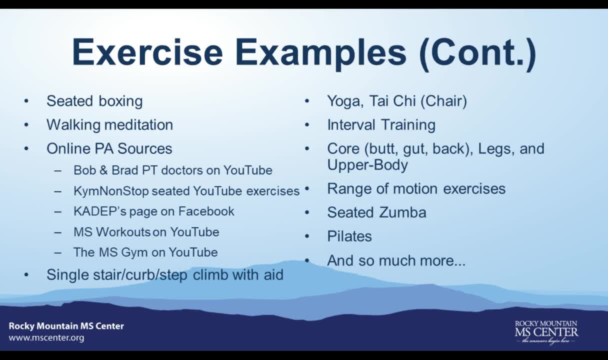 And based on one of the comments in your webinar, I have a feeling these two questions are linked. One person asked what are tricks nutritionally to boost your energy- Energy to exercise- and somebody else asked best ways to reduce belly fat if you can't do intense cardio. 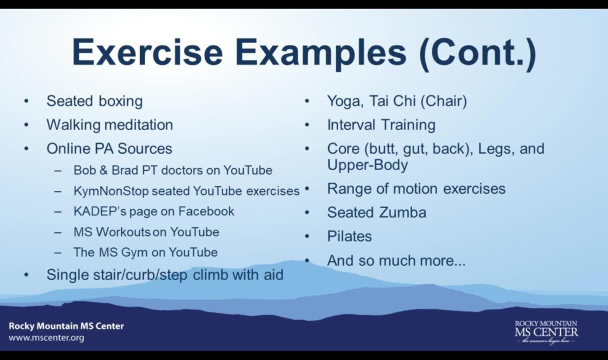 So boosting your energy to exercise and then ways to reduce belly fat. So when, when it comes to mind for energy is working out, when you get up and you, you know you've had your rest and then you can jump into an exercise routine and then go, you know, preferably then still be able to go on your day. 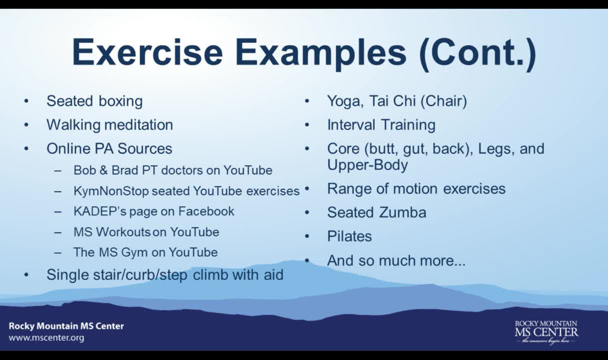 But working out after sleep is actually something that athletes do. They'll take a nap before they, before they get going, just to help give them some more energy To get there, though you might have to again start start with instead of going right to 30 minute sessions. 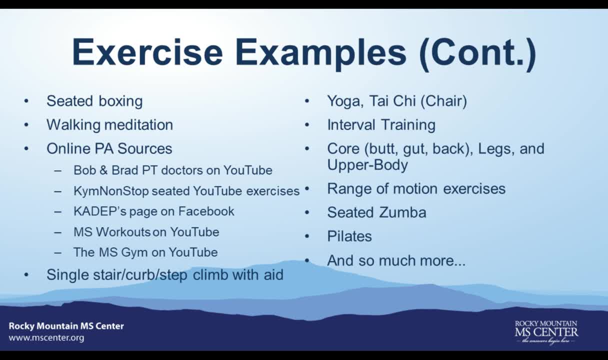 doing, you know, five or 10 minute sessions and starting out there and working your way up. That is. that is kind of what it would one one way that it would take to help you boost your energy for exercising. starting small again. 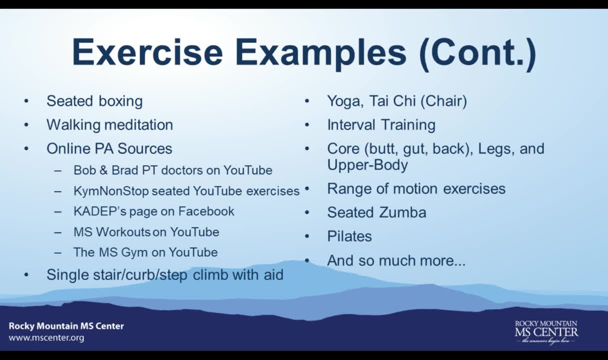 And then, in terms of helping with belly fat, there's you know, you could, you could do all the the crunches and and everything. That's not going to quite help you get rid of your, your fat entirely, though. 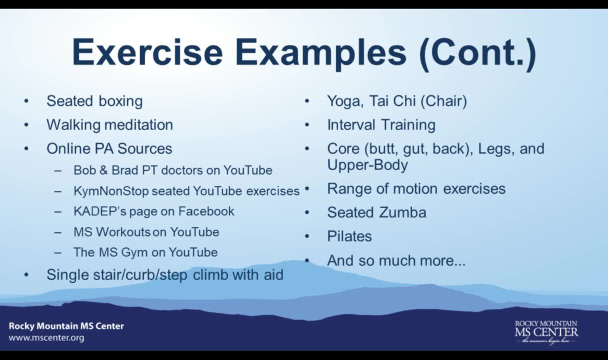 It's. it's important In terms of a caloric standpoint just to be able to burn the calories that you consume, but there's one way to help you get rid of some of your fat and and those calories and you need to consume a little bit less. 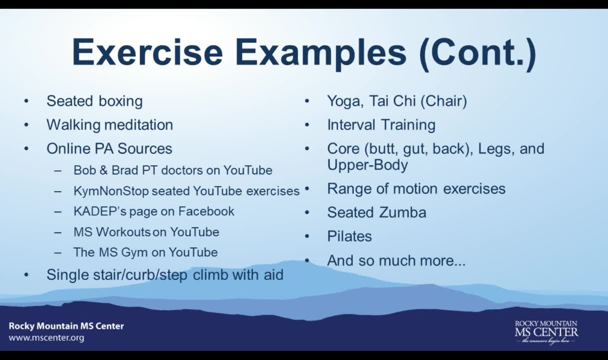 If I'm talking ever about dieting or nutrition, better yet I'm. I'm always emphasizing muscle and as well as as having a balanced diet. Don't just be consuming carbs or proteins all the time. You know, get, get your vegetables in there, of course, get your your irons still, get your proteins and and your potassium and everything else that you, you know you you should have, but also do it in moderation. 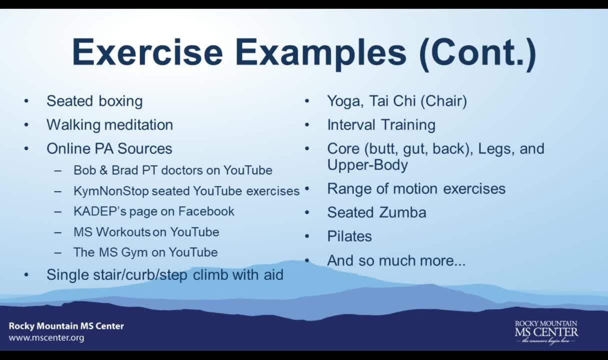 So a balanced diet, in, in moderation, that's. that's the best I can tell you in terms of starting on a path to getting rid of your belly fat, and from there then it's kind of about also putting in a little bit extra activity and building yourself. 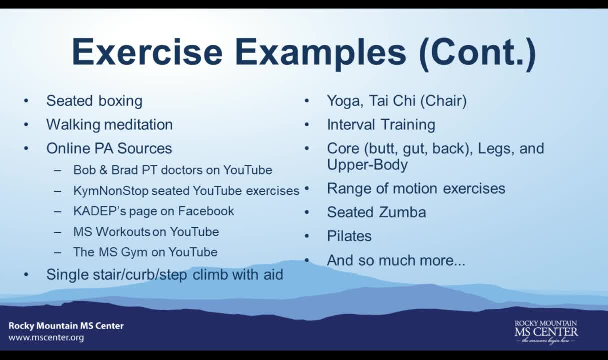 To that, that level that it would take to for your fat to start burning off a little bit more. taking taking both those into account: first the dieting and then the exercise- Awesome, I think that is all that we have time for today. 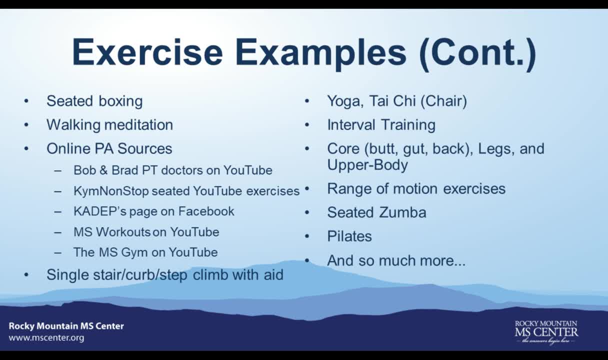 So thank you, Ryan, so much for your time today and sharing your expertise for everyone that questions. We got one more question in. if you have a quick moment, Sure, Do you have any good stretching programs or props, Or what was that?